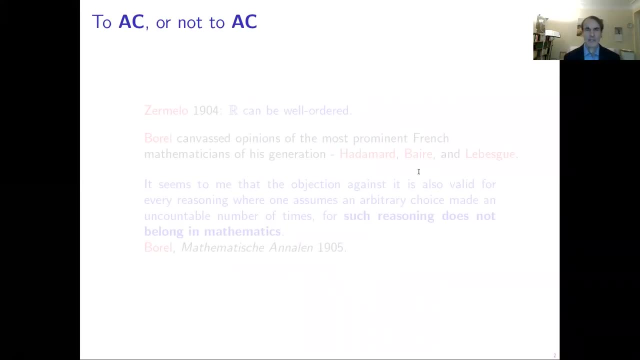 Okay, So the question of to AC or not to AC was important at the beginning of the 20th century. Zermelo had proved that the reals can be well-ordered, And then Borrell canvassed opinions of the most prominent French mathematicians of his generation. 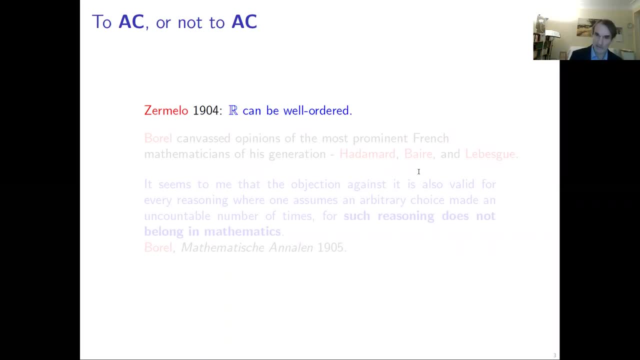 including Adamas, Baer and Lebesgue And so. So this was the upshot of it. There was some. He published something in the Mathematische Annale in 1905.. It seems to me that the objection against it is also valid for every reasoning. 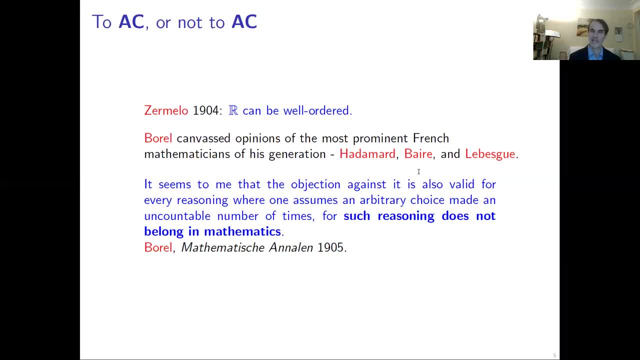 where one assumes an arbitrary choice made an uncountable number of times for such reasoning does not belong in mathematics. So very strong rebuttal of the axiom of choice. The opinions of Adamas, Baer and Lebesgue were that okay. Adamas sided with Zermelo. 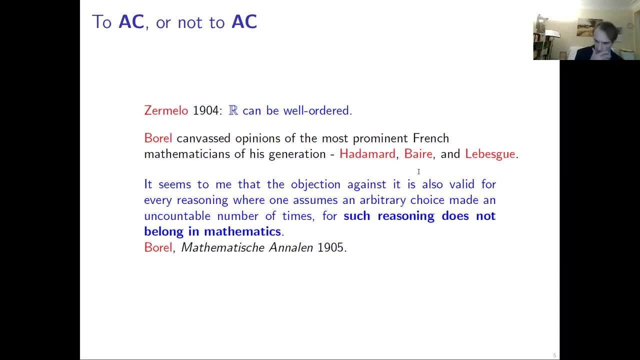 whereas Baer and Lebesgue agreed with Borrell. Okay, So the question of AC. Hilbert, of course, suggested another way of dealing with it, namely not to view it as a metaphysical question, but just to see what can you do with AC? 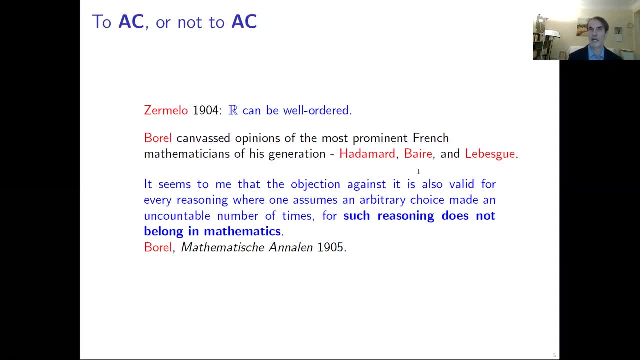 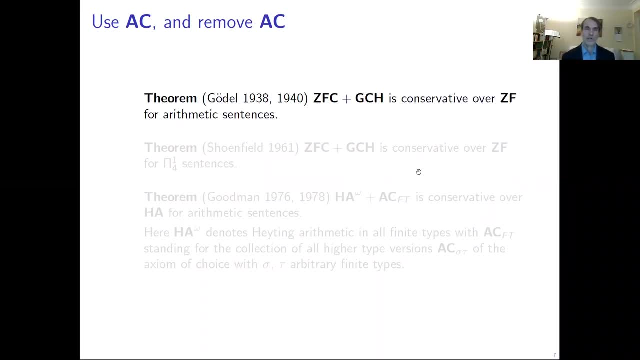 and maybe you are able to use it as an ideal element which can be eliminated afterwards. And So in classical set theory we know that if we add the axiom of choice or even the generalized continuum hypothesis, this will be conservative over ZF for arithmetic sentences. 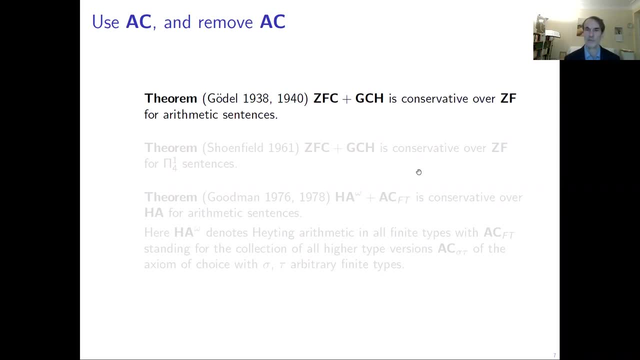 So Gödel used the constructive hierarchy, of course, and you can even go further in the Schoenfield via the Schoenfield absoluteness lemma, which showed that Basically you can go up to pi 1, 4.. Okay, In the constructive world. 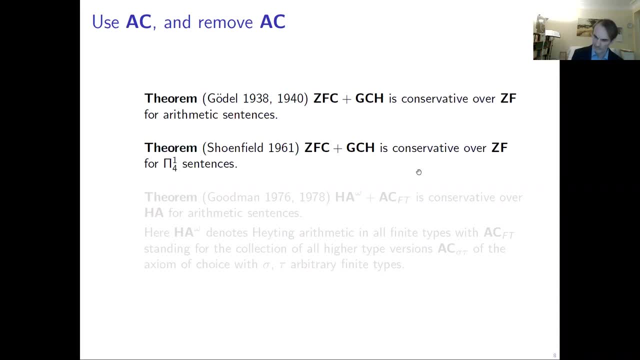 if you deal with intuitionistic theories, the situation is a little bit more complicated. So the proof that ZFC is conservative over ZF for arithmetic sentences just follows from, yeah, the constructive hierarchy. In the realm of constructive theories. there's a famous result due to Goodman. 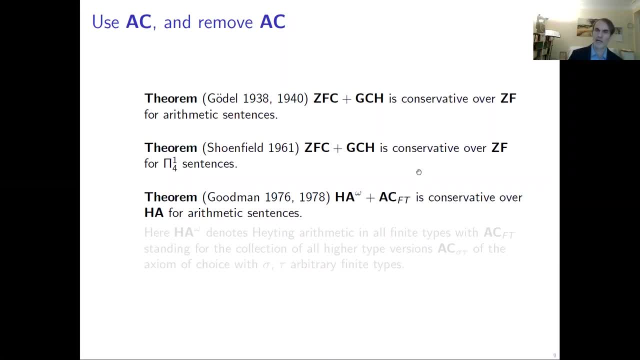 So if you look at Heighting arithmetic, By the way, can you see my? Can you see the cursor move around something? Yes, Yeah, Yeah, I saw this. HA omega stands for Heighting arithmetic in all finite types. 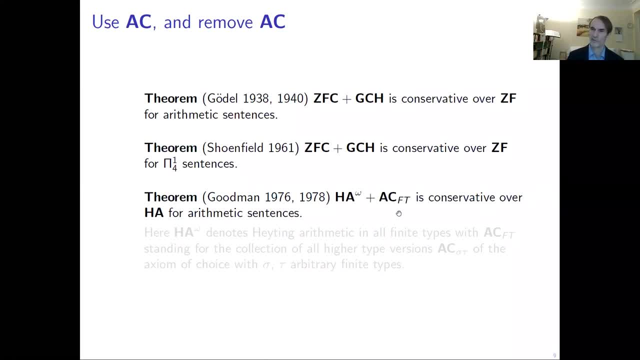 And then you can add the axiom of choice for all of these types, And Goodman showed that this is correct. He showed that this is conservative over HA for arithmetic sentences, And the proof is rather complicated and he had two approaches: one via his theory of constructions. 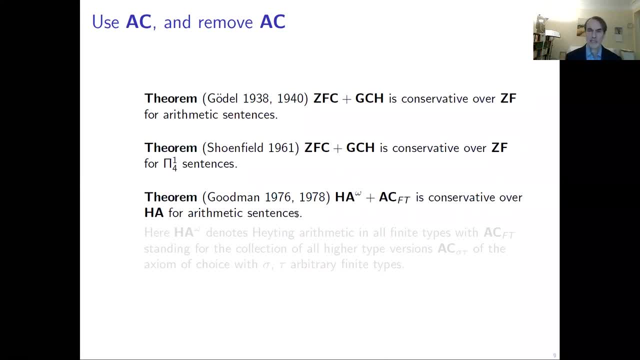 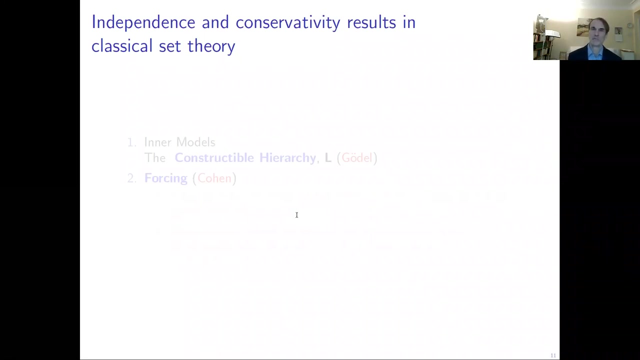 and later a nice way of slicing the proof into two parts, namely one part being realizability and another part being forcing. Okay, I will define these axioms, AC sigma tau, later Now. in classical set theory, we have several tools for showing independence. 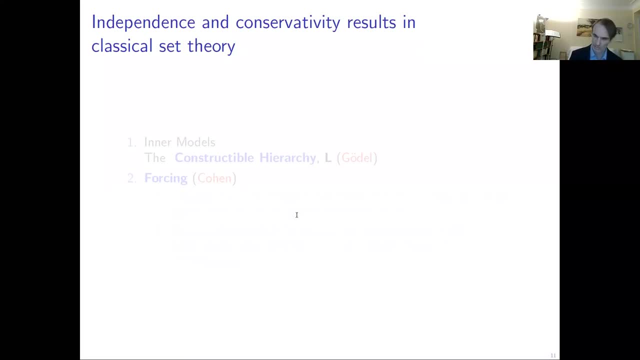 and conservativity results. And one is the inner models, for instance L, and another one is forcing Permutation models as well. Now, going to the, The intrusionistic world, one might also look at the constructible hierarchy. So now I'm looking at basically. 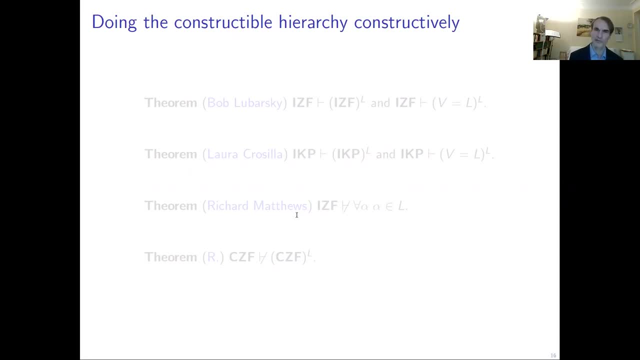 intrusionistic set theories. So IZF stands for the intrusionistic version of IZF Of Samuel Frankl set theory, And you can do the constructible hierarchy constructively. I'm just stealing a title from Richard Matthews while ago in Leeds, And the result is that 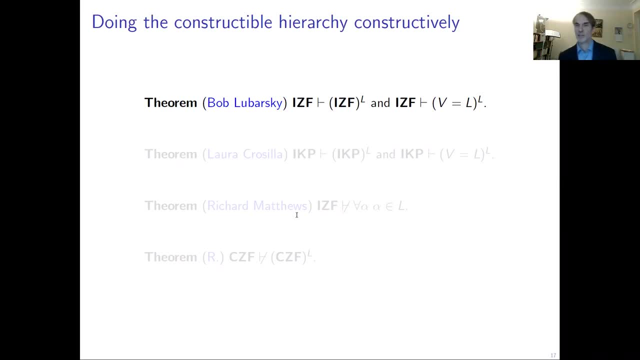 well, the constructive hierarchy also works to some extent, Namely on the basis of IZF. you can show that L is a model of IZF and you can show that in L, V is the same as L. Also, this was done by Laura Priscilla. 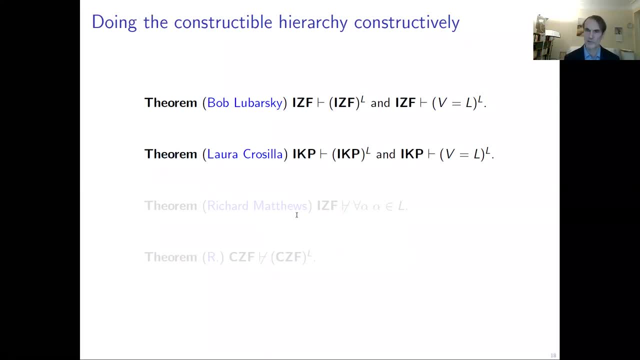 so she looked at this in the in the case of Kripke-Platek. So the endogenous version of Kripke-Platek set theory, the same obtains there. But then also Richard Matthews showed that L is a somewhat unregulated. 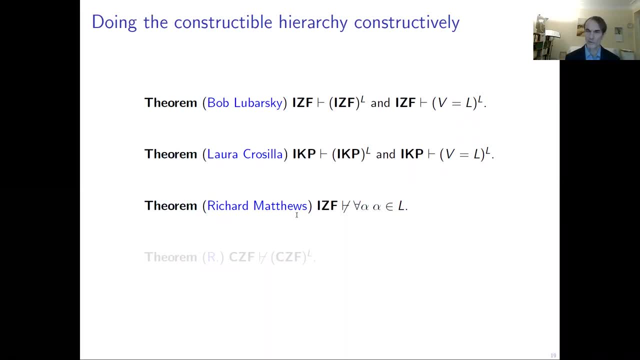 entity in the endogenous world. So you cannot show that all ordinary, those R and L. And finally, it can also show that when it comes to constructive Samuel-Franco set theory, that constructive Samuel-Franco set theory cannot show that its 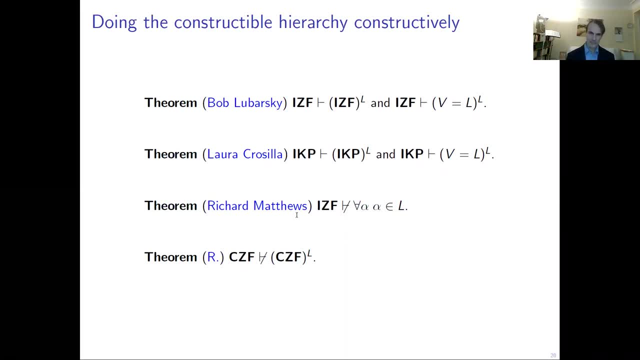 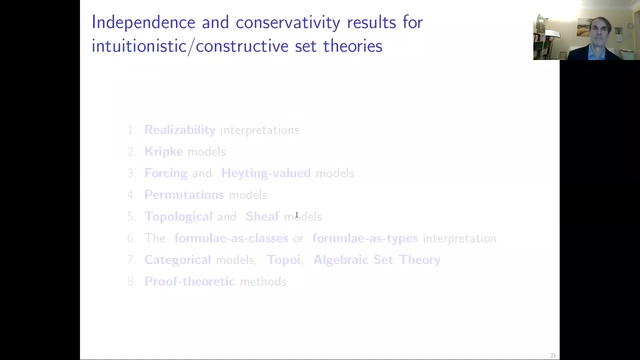 axioms hold in the constructive hierarchy. So it turns out that this is somewhat you can do the constructive hierarchy, but it's somewhat useless in this context. In the realm of interesting theories, you have many tools to show independence and conservativity. One of the 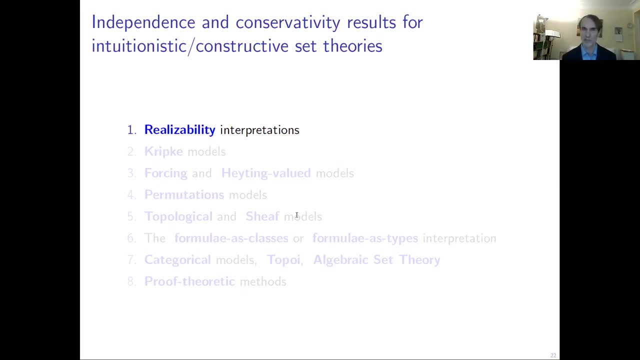 oldest and most successful, perhaps, is realizability. And then there are lots of other methods. You can, of course the Kripke models, forcing and hiding valued models, So the interesting theory can be used to show that there's an interesting version of Boolean valued. 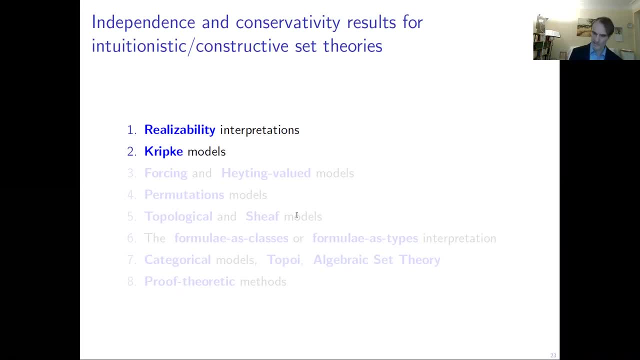 models. that also works for intuitionistic theories. And there's many more tools like sheath models, topological models, categorical models and also proof theoretic methods, But today I will just use the oldest method: realizability. OK, just a brief. 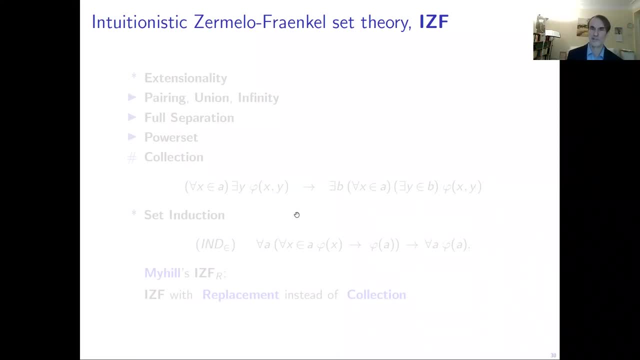 look at the axioms of IZF. So this is the intuitionistic version of the IZF, which is the version of ZF, And so we have the same many times. we have the same axioms: extensionality, pairing, union, infinity, full separation, power. 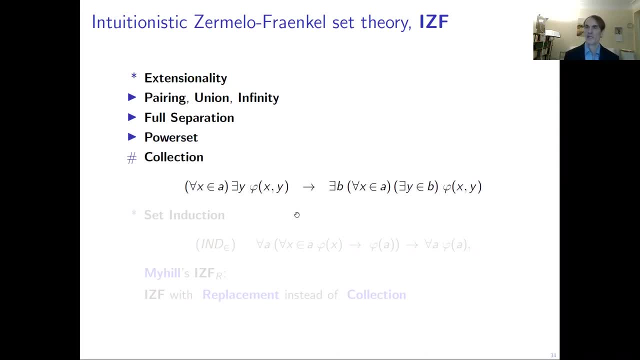 set Instead of replacement. replacement is somewhat awkward, intuitionistically. Instead of replacement, one uses a strengthening collection Instead of foundation, one uses the positive set induction scheme And that's it. So, basically, the idea is one makes, one changes the underlying logic of ZF and makes minimal 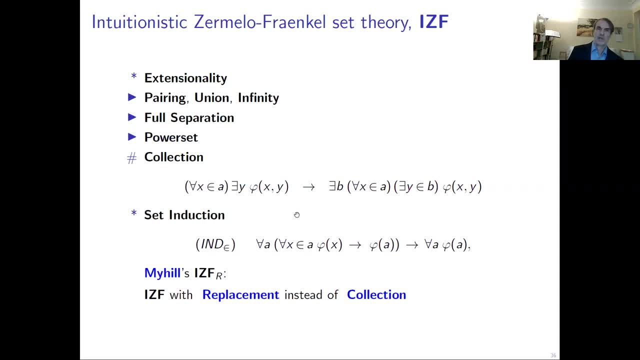 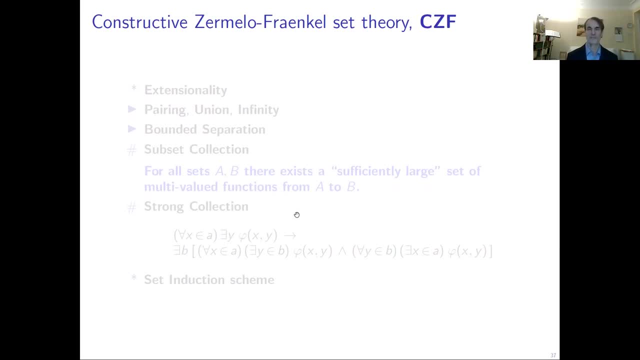 changes. I already talked about constructive Sarmiello-Fraenkel set theory, CZF. This is a set theory which was first proposed by Myhill as a background system- background framework from constructive mathematics- And then later Peter Axel wanted to connect it to. 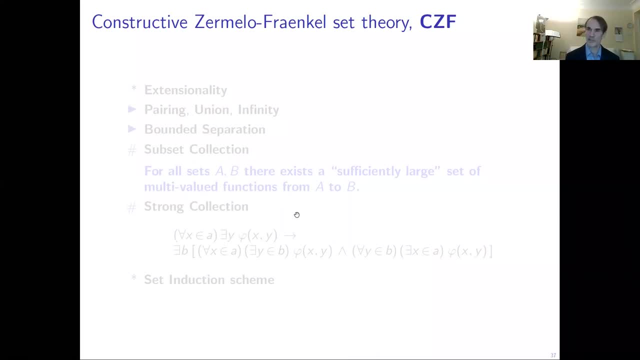 Martin-Lev type theory And he defined an interpretation of Myhill system in Martin-Lev type theory And he found that some of the axioms can actually be expanded. OK, so CZF has extensionality, pairing, union, infinity. as before, Separation is a. 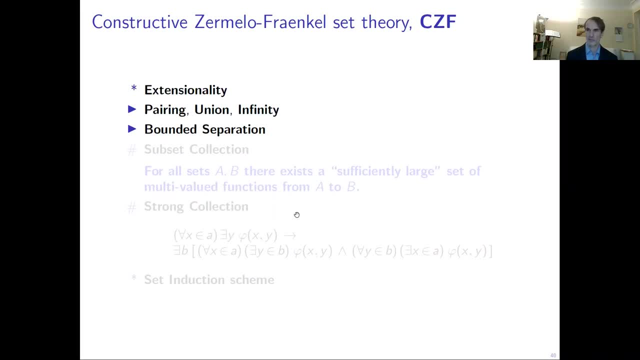 restricted. So bounded formulas just to bounded formulas, where bounded formula is one where the quantifiers appear as for all, x in A and there is a y in B. only in this restricted form, Instead of power set, one has subset collection. This is an extension. 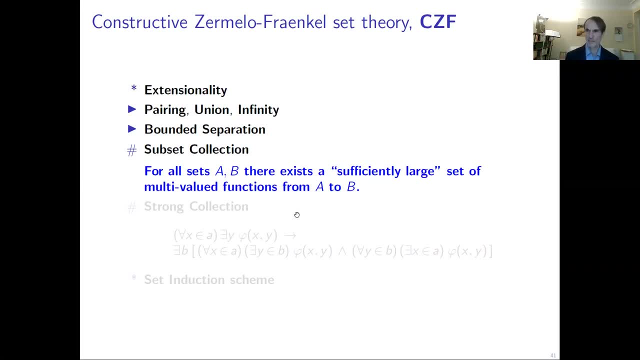 basically of Myhill's axiom called exponential set. This is an extension. namely, if you have two sets, A and B, then the collection of all functions from A to B is a set, And furthermore, CZF has an even stronger collection. 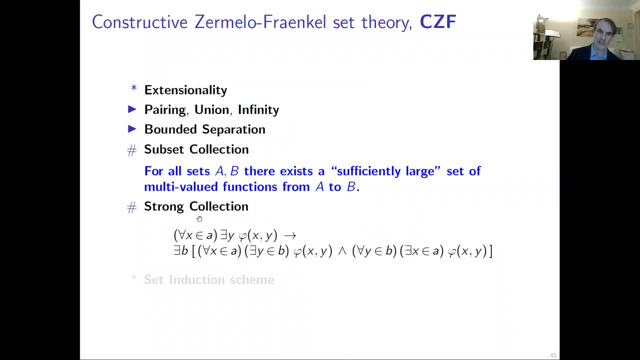 scheme. So you have the same premise as in the collection scheme, but then the conclusion is stronger. So in collection you basically find the B so that you can collect that you have enough witnesses for these y's in B. But since you lack, 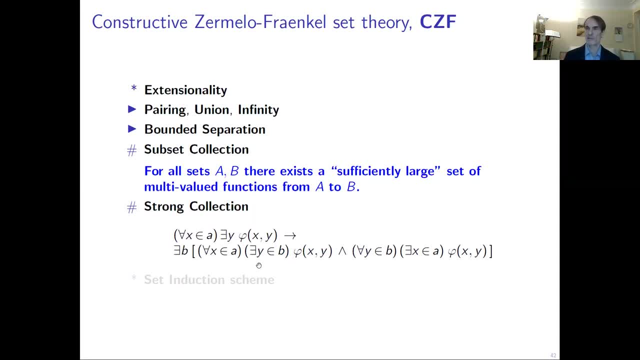 full separation. this can be sometimes not a very useful set. So the strengthening is that this B consists of witnesses y for the x's in A, but also vice versa. Anything in B comes from some x in A, so that phi x y holds, And then you have the 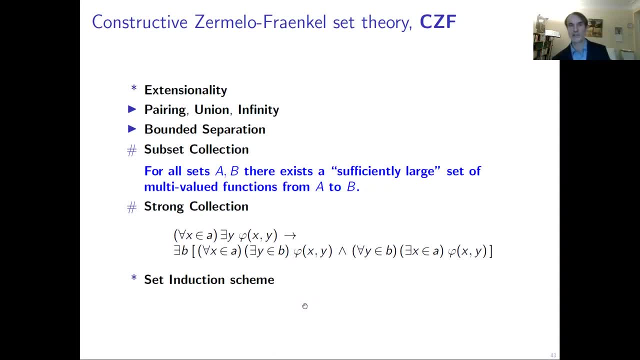 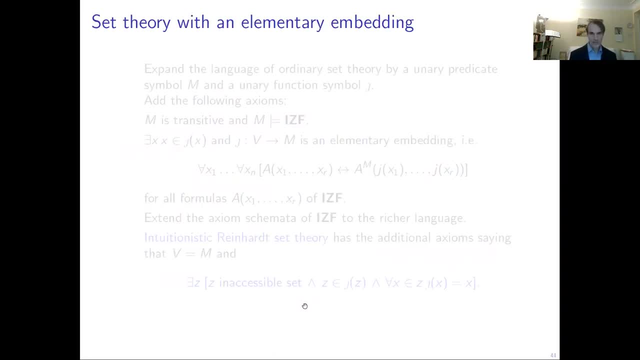 reduction scheme. OK, so these are the two main theories. One is interested in interstitial context, But you can actually go way beyond that. For instance, you can study large cardinals. Well, they are not large cardinals, They are large sets. here. 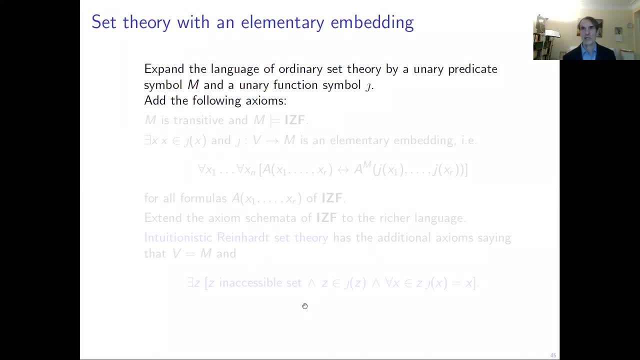 So you can add sets asserting where the sets are inaccessible or where the sets are malo, And, for instance, you can also expand the language to accommodate elementary embeddings in the interstitial context. So if you add, for instance, the symbol m and the symbol j, 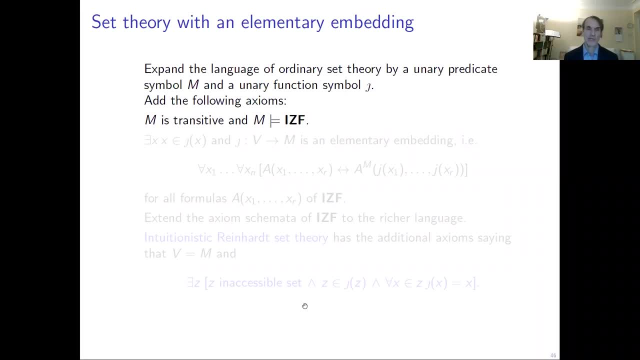 so j a function symbol. you can express that there is an elementary embedding. So if you add these accents here, so the m, you say that m is a transitive class. So if you add these accents here, so the m, you say that m is a transitive class. 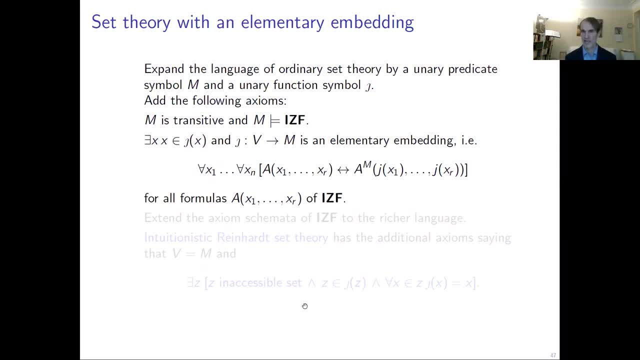 So if you add these accents here, so the m, you say that m is a transitive class And all the actions of IZF hold relativized to m. And with regard to j, the elementary embedding, where you say it's non-trivial, so there is an x, so that x is in jx. 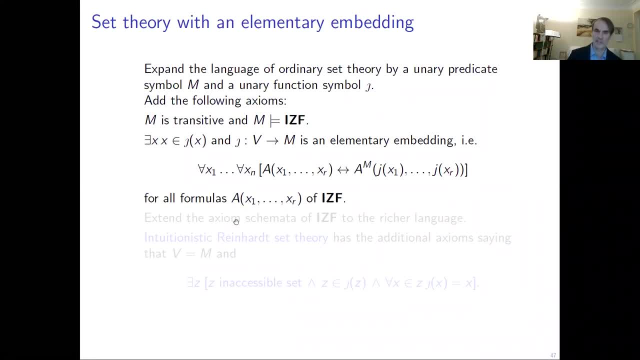 And it's an elementary embedding and you express it via this scheme here, where the formula a here is from the original language of IZF, so it doesn't contain j and m. So a formula ax holds if, and only if, ajx holds. 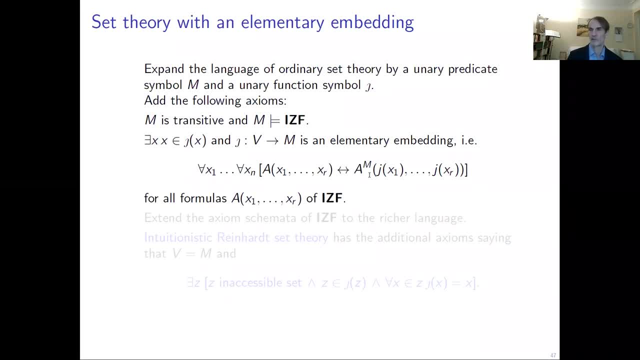 but a has to be relativized to m, So all the quantifiers have to be relativized to m. That's what it is. And then you can express something like intuitionistic, say, Reinhardt set theory, And you can also find counterparts to. 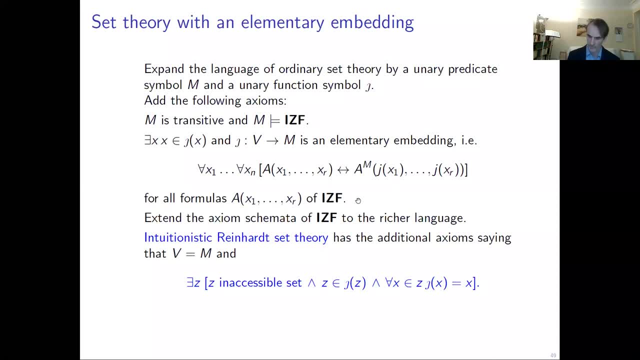 like super compactness, hugeness and so on, Right. So all of these intuitionistic set theories are also interesting to study. And these days it might be even more interesting because, as you perhaps know, some researchers in set theory have studied even extensions going beyond Reinhardt. 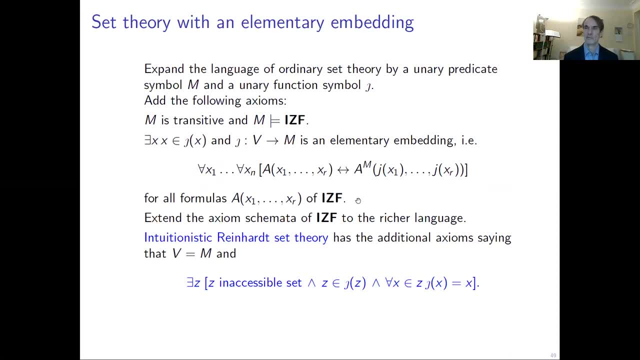 like Berkeley Cardinals and so on. It is known that in that context you cannot have the full axiom of choice. Yeah, Because it gives an inconsistency. And so it might be interesting to study the intuitionistic counterparts of these classically very strong and actually intuitionistically. 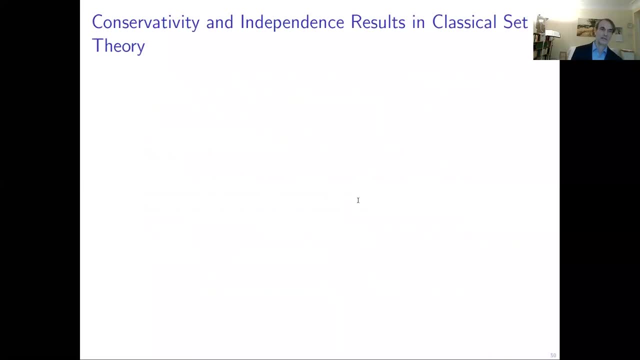 also very strong set theories. Okay, Oh, This slide the one in between. I did not want, Sorry about that. Okay Now, I said today the main tool, the main tool will be a Kleene realisability. Well, actually there are lots of different kinds. 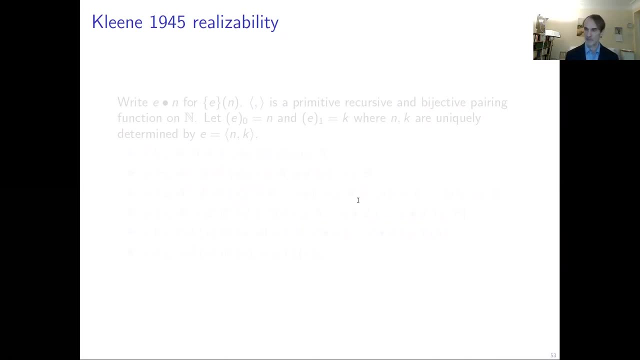 of realisability, And the first one was started by Kleene, And so in 1945, he gave a realisability interpretation of heightened arithmetic And okay, So the idea is here. you use, let's say, programs E for Turing machines. 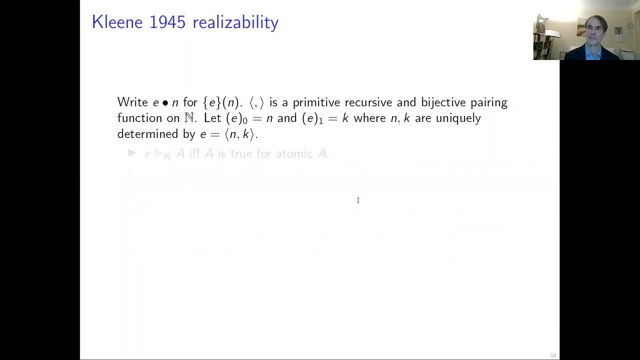 or let E can be the well. you have a listing of the partial recursive functions. So E is the E's partial recursive function, And then, with these partial recursive functions, you do an interpretation of intuitionistic logic which very much resembles the so-called 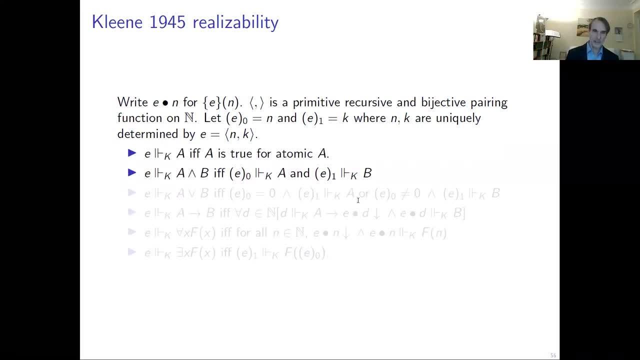 Brauer-Heitling-Kolmogorov interpretation. Okay, Let me just point out the interesting bits. So in the case of disjunction- so E is a realiser for a disjunction, Well, E has to decide which of the disjuncts. 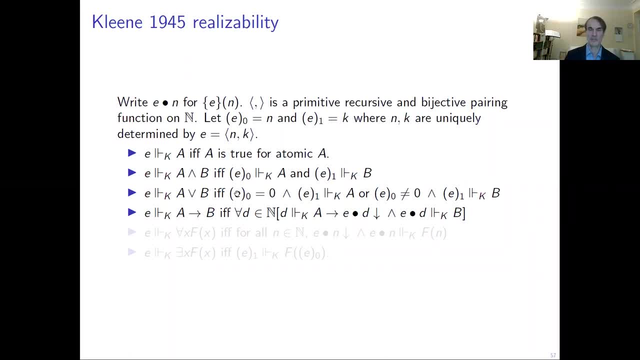 it wants to realise. If the first, so this E, can be decoded, okay, there's a projection function. So if the first projection is zero, then the second projection should be a realiser for A, And if the first projection is not zero, 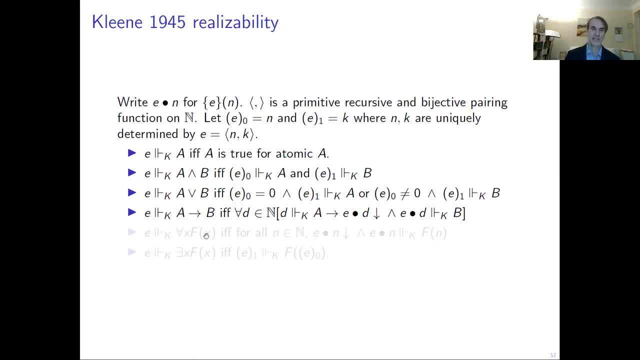 then the second projection should be a realiser for B. And then the interesting cases are implications. So it means that E realises an implication. if whenever you have a realiser for the antecedent, then you apply E to this realiser. 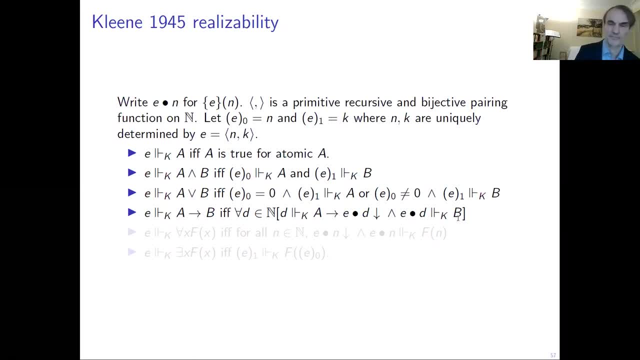 and get a realiser for the succedent of the implication. And in the case of quantifying, well, it means that E realises a universally quantified statement if, for each natural number, n, E applied to n is a realiser for the instance f of n. 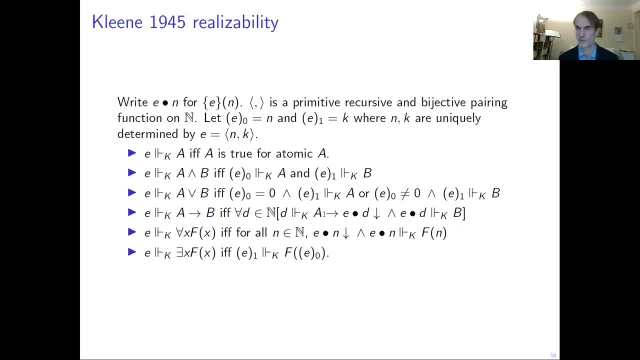 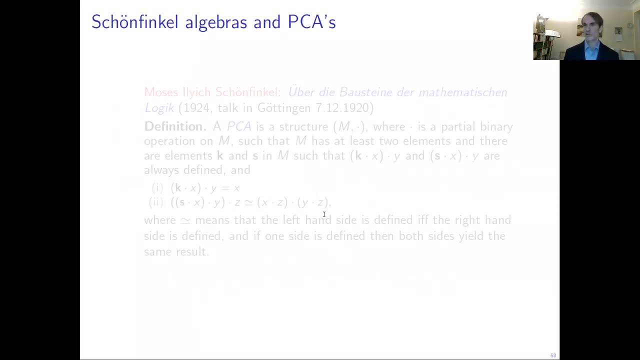 Okay, And in the case of the existential quantifier, the realiser is supposed to provide a witness. So this is very similar, as I said, to the BHK interpretation. Now, the realisability that Kleene used, the first one, was basically what's called K1.. 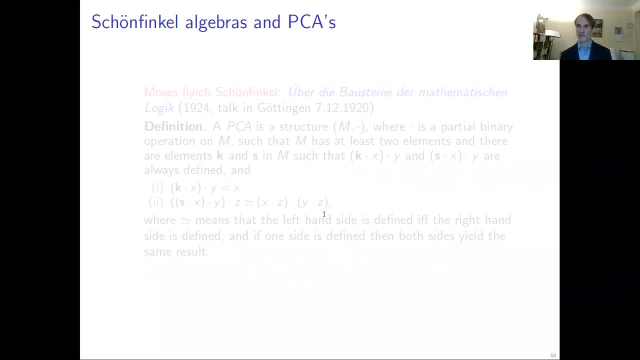 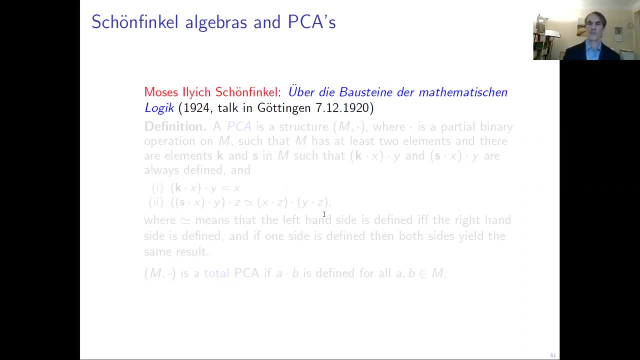 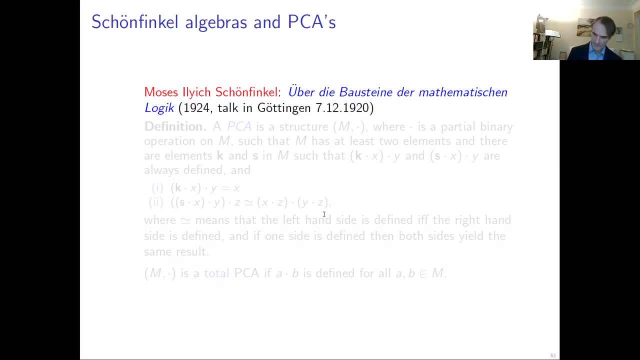 So he talked about, which means about, on the basic building blocks of mathematical logic And applied in fields in different dimensions, in linear logarithms, and so these structures, These structures are, at least days, called Combinatorial Algebras or Partial Combinatory Algebras. 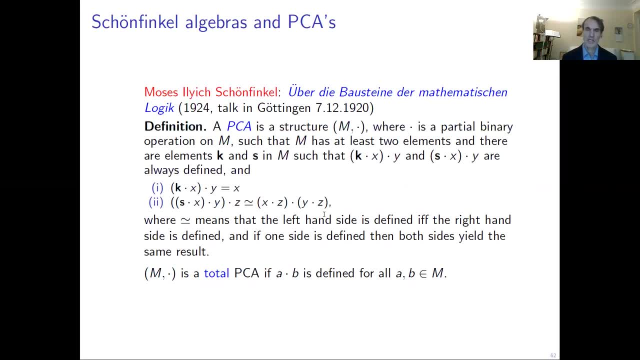 over which you can do computations, And so these kind of combinators, as they were called later K and S, were already identified by Schoenfinkel. And so what you have here, PCA, is a structure M with a partial binary operation on M. 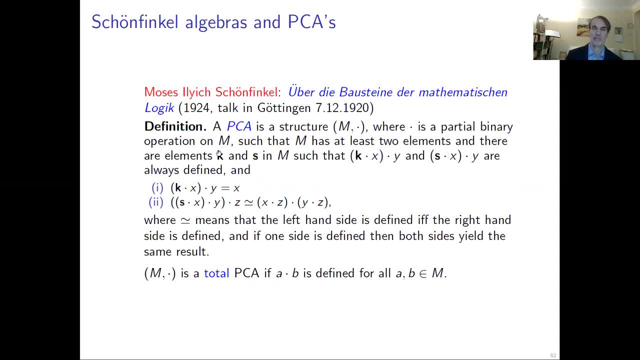 and there are at least two elements in it: a, K and S. And the thing is that if you first apply K to X- this is always defined- and then apply the results to an arbitrary Y, you get X back And the other S. 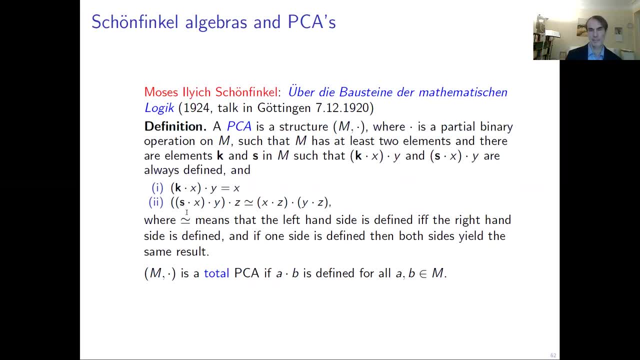 what it does is if you apply S to X and we apply the result to Y and then apply that result to Z, if it's defined, it's the same as the first: apply X to Z and then applying Y to Z and then applying the first result to the second result. 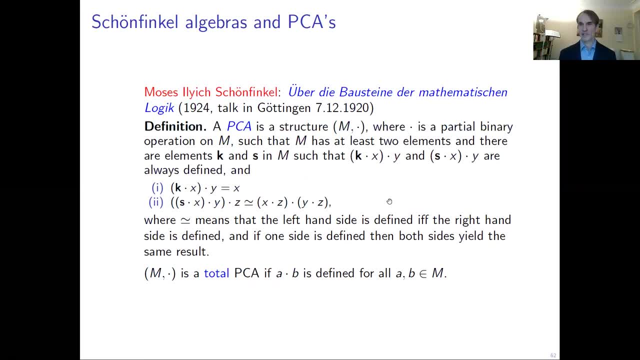 And these are structures. this is enough basically to do a nice theory of To do computations. Actually, Schoenfinkel did only the total case where you have a total, partial, binary, operational M. The partial case, I think, was only identified much later. 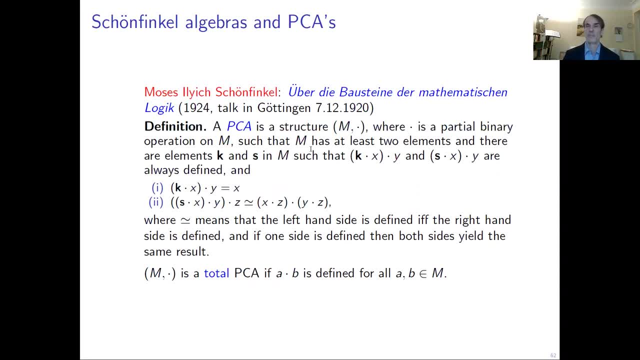 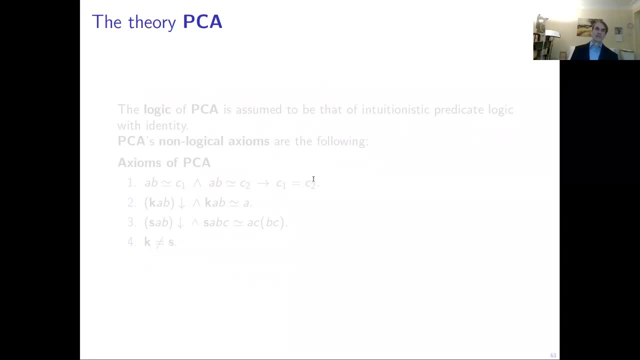 though it could have been actually identified much later. though it could have been actually identified much later, could have been identified very early on, and I think it was Pfefferman who first used the partial case. okay, and we can also make a theory of from these structures also called PCA and has the obvious 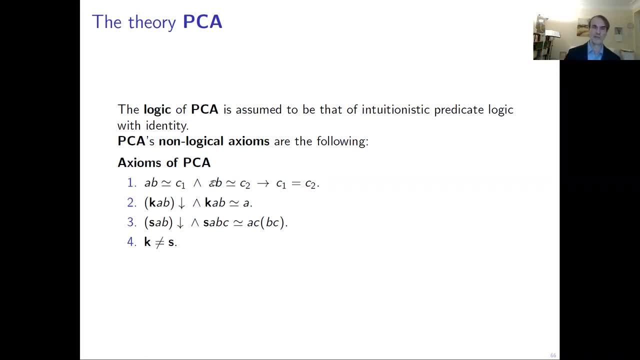 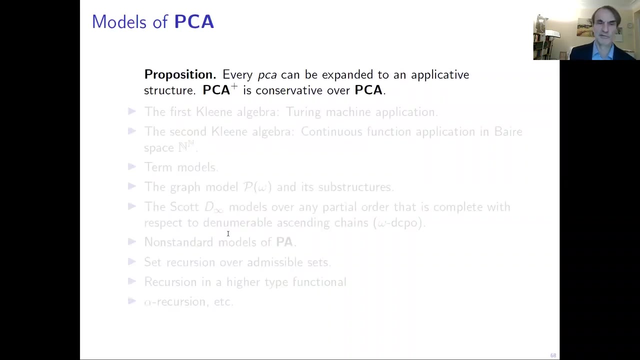 axioms. and here I omitted the dot. yeah, so the convex is really that the dot, the operation, is omitted. just write the terms without the dot, okay. and there are lots of models, lots of PCAs. just one remark: very often one looks at so-called applicative structures. these are 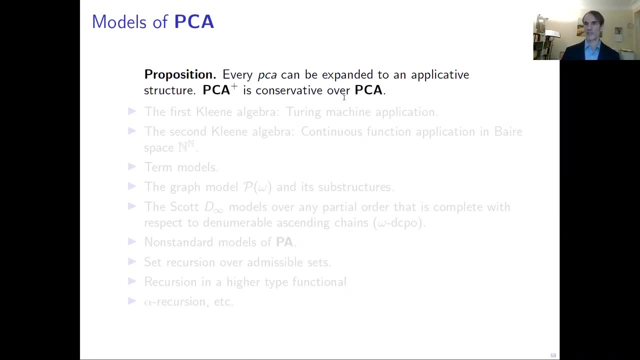 a bit richer. but basically you have a copy, you identify a copy of the natural numbers and you do case distinction on the natural numbers. but it turns out that any PCA can be expanded to this richer applicative structure. okay, so what are examples? well, the first, cleaning algebra, is where the operation is Turing machine application. 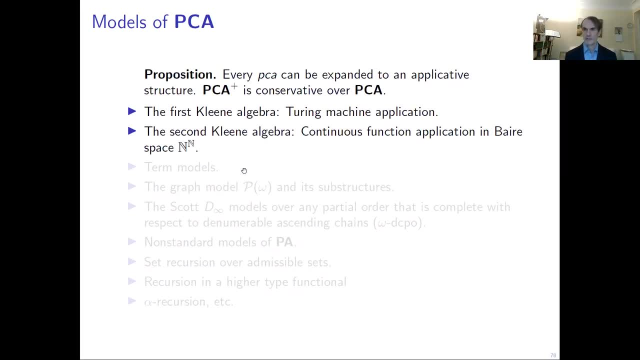 the second cleaning algebra. here the underlying domain is bare space and what you do is the operation is continuous function application. and then there are lots more, there are term, and then there is also the Schrodinger one and then the other one, two point terms that are expected to be transformed as차�ics. and then we can take just three cases and then we can do a set recursion of admissible sets. basically, any notion of computation gives rise to a PCA recursion and higher type function of alpha recursion and so on. so this is a very rich collection of structures, a lot of data into this case, because apparently if you can take a lot of data into a set recursion which can be easily eliminated- but that's not the main point of this project- 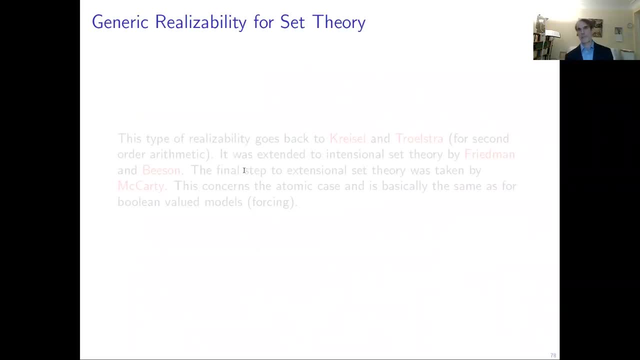 And now I would like to come to the main technical tool. This is realisability, as I said before. But this kind of realisability is strikingly different from Kleene's 1945 realisability And, okay, I gave it the name- generic realisability. 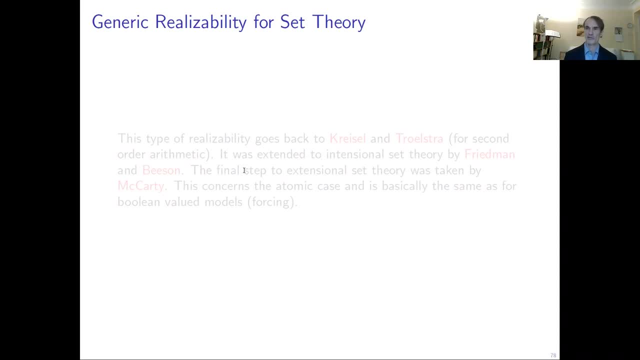 And this is actually this terminology I think is due to David McCarty, And I'll explain soon what I mean by this kind of genericity. It's not the genericity usually related to forcing. Okay, so this type of realisability historically goes back to Kreisel and Fulstra. 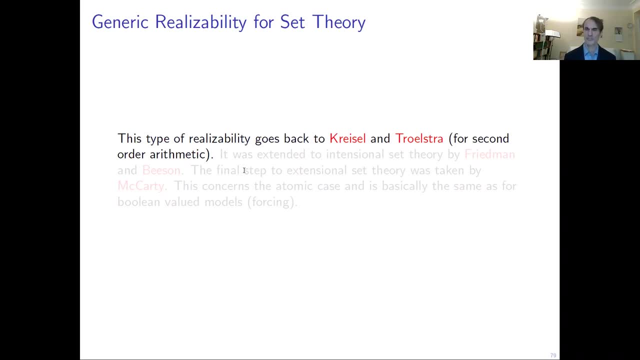 They used it for second-order arithmetic. It was then used for set techniques. It was used for set theories, for intuitionistic set theories. Well, I call them here intentional set theories, by which I mean that you just don't have the axiom of extensionality. 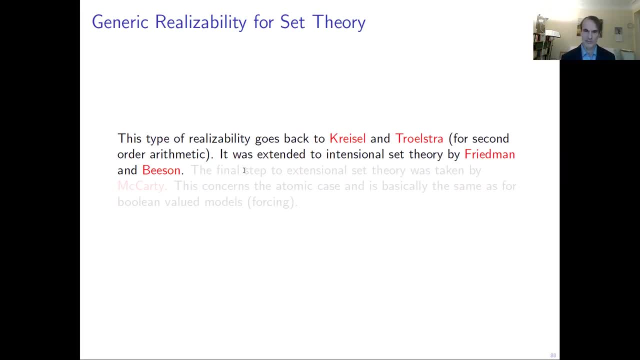 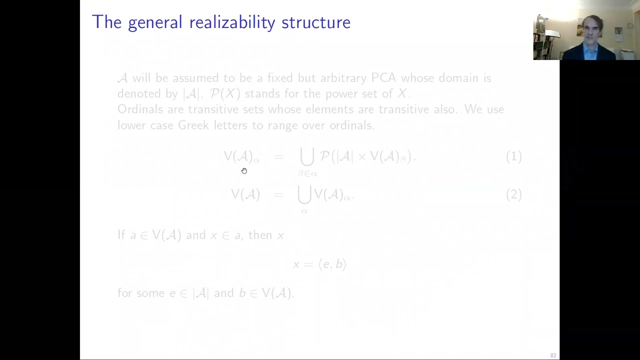 And then the final step was done by David McCarty, So he then transferred it to extensional set theory And it's basically that the atomic case is dealt with like you do in enforcing or Boolean-valued models. Okay, So to do realisability for set theories, one starts with a PCA A. 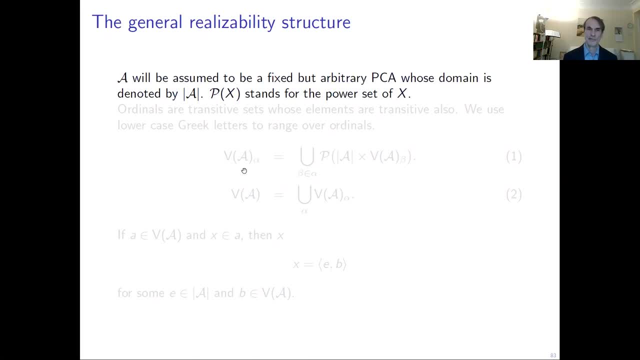 Okay, And then from the PCA one generates a universe as follows: So the stages of this universe are denoted by VA- alpha. And so here you see. what happens is that going to VA of alpha means you assume you have already defined VA of beta for beta less than alpha. 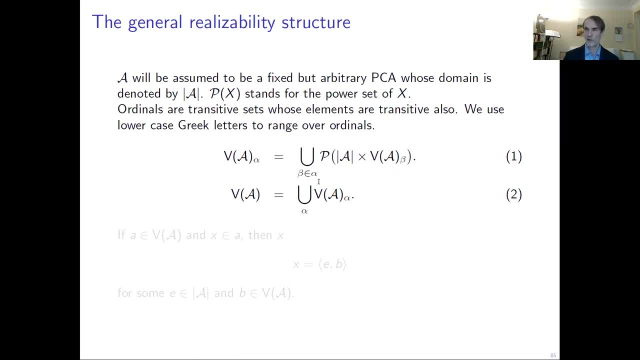 So in intuitionistic set theory the ordinals are defined in the same way as classically: Ordinals are transitive sets whose elements happen to be transitive sets, But of course you don't have linearity as in the classically case. 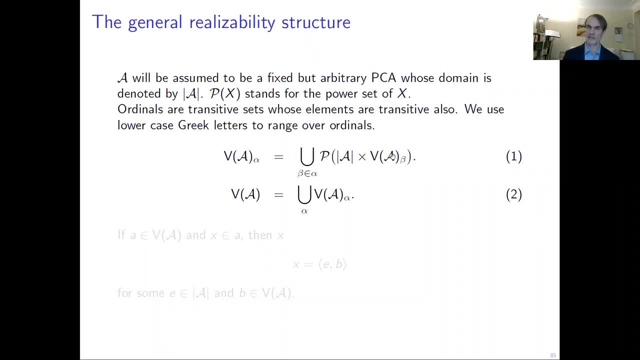 Okay And then. so basically you have already defined the chunks VA beta for beta in alpha, And then you take the power set over the domain of A times VA beta for all these betas, Then you union them up And that's your VA alpha. 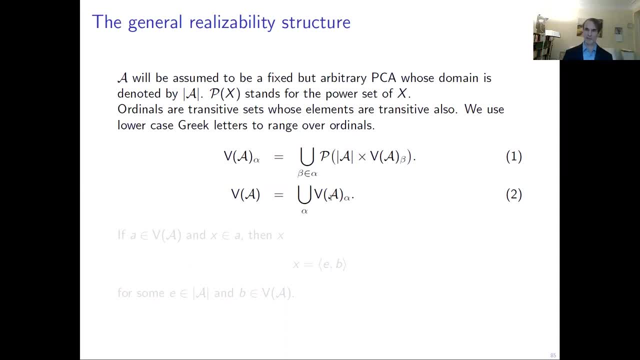 And then the whole class structure for realisability. VA is just the union of all these VA alphas. To look at this a little bit, how do the elements of this realisability universe look like? So if you take an A in an element of VA and you take an X in A, 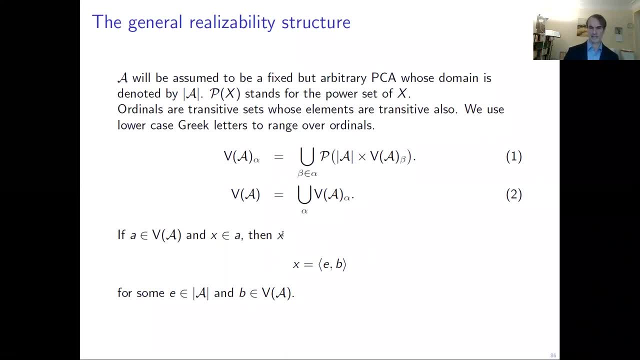 Well, how does it look? Okay, So this is what it looks like. Well, this X is going to be an ordered pair, where the first component is E, belongs to the PCA, A, Yeah, And the second component is just another denison of the world, VA. 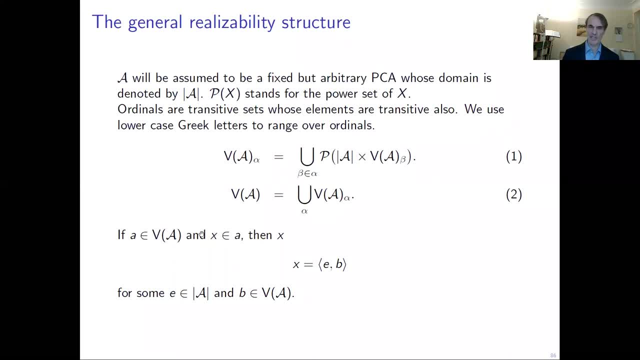 The thing is that these elements of A, they come equipped or tagged with some extra information from the PCA, So some kind of computational information here on which certain realisers from maybe the object, the elements of A, can act. Okay, So that's the realisability structure. 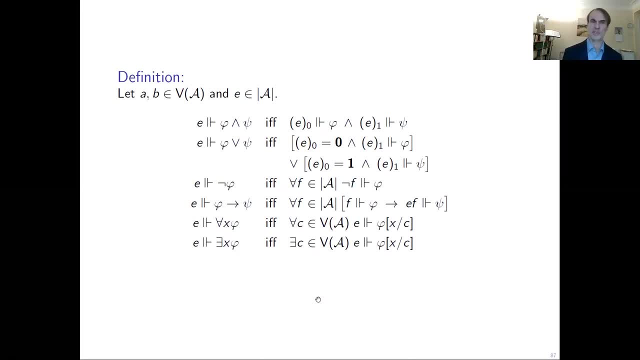 And then you define a notion of realisability. So the realisers are elements of the PCA, And then it's the realisability. Well, in the beginning it goes very much like this: It goes very much like in the Kleeney 1945 realisability. 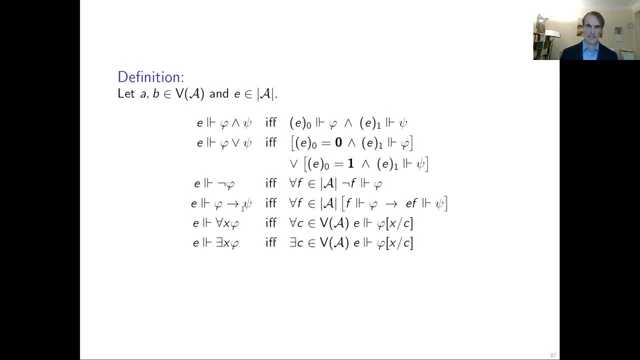 This definitely applies to and or and to implication. But then we come to quantifiers and, you see, something surprising happens, Namely what is a realiser for a universally quantified statement. So this is a statement over all sets. 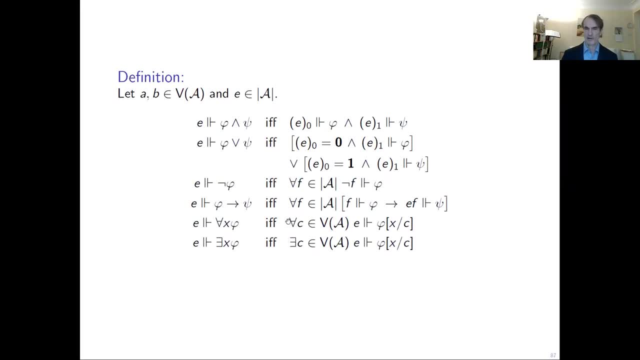 Yeah, And this means that for each individual C from the realisability universe E realises. And now you substitute this C for the X and phi And you see what happens is sort of the E here. the realiser doesn't take the C into account. 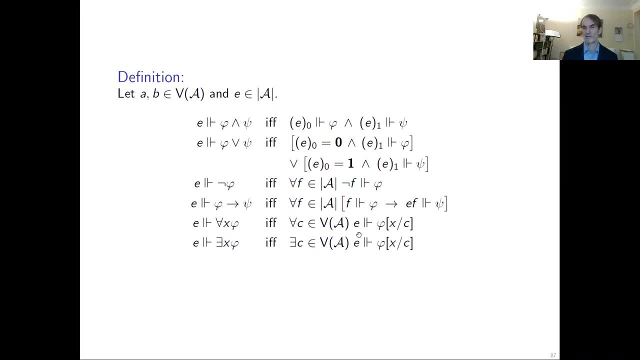 It doesn't act on the C at all, It's kind of, it's a realiser for every instance And this is the reason for giving it a name, The reason for giving it the name generic. So it only looks at these objects in the in the set theoretic world VA as generic objects. 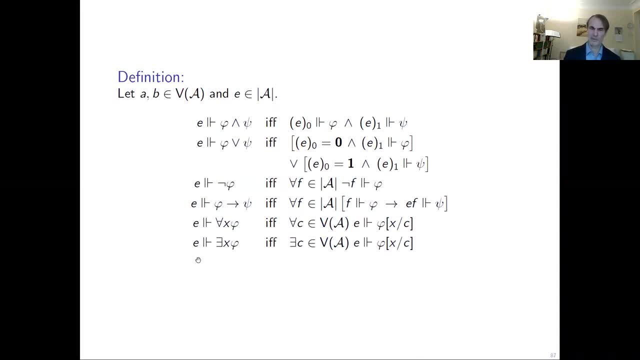 Okay, And the same applies to the existential quantifier. Yeah, Just the realiser just marches through. So it just means there is a C in the in this world, so that E realises phi of C. So it's kind of a surprising kind of realisability. 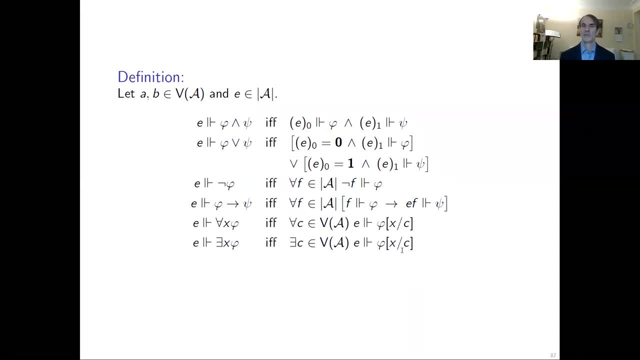 If you think about it, you will also realise, actually, that it wouldn't be possible in any other way. because, well, if I were to do this in, like in the Kleene case, then this realiser E would have to entail a witness for this C, so that phi C holds. 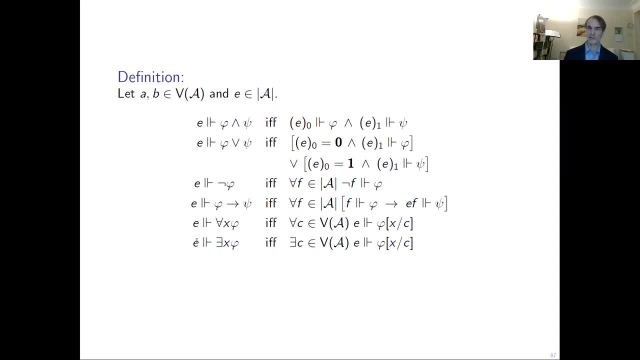 But you know, in a universe and this realiser, if you want to realise maybe a large set, X, and that there exists an inaccessible, then it wouldn't be possible if you did it in the Kleene way, because these E's here are from, they come from the PCA and they cannot contain this huge object. 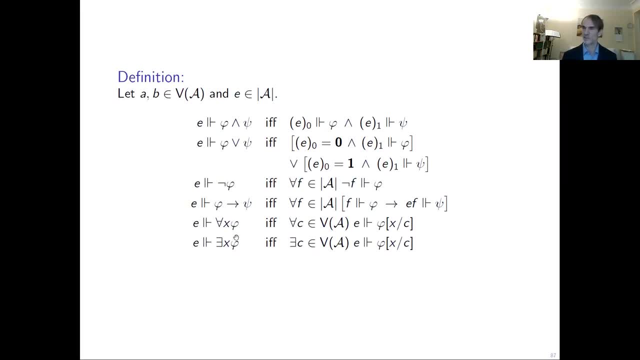 So it's something that's clear that it has to be done in this way, but it's surprising that it works. Okay, Now the atomic case on the previous slide. the atomic case wasn't there, All right, How's that done? 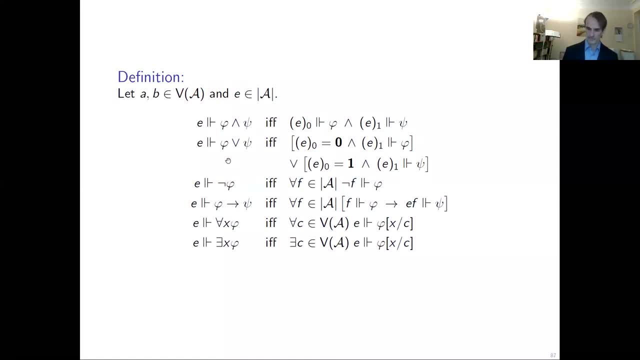 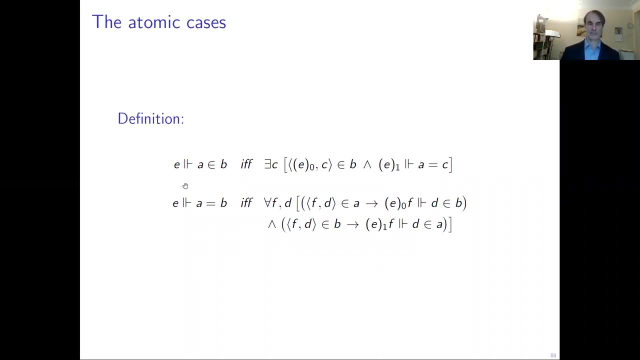 Well, the universe is built up inductively, Yeah, And you have to follow this build up. And so if you have two, if these two objects- AB, belong to the realisability universe, VA, then E realises A as in B. if 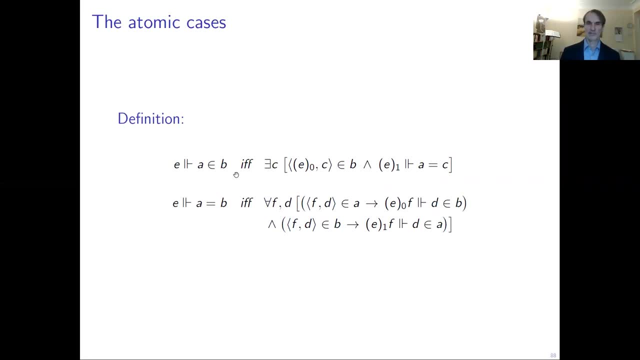 Well, remember that the B, the elements of this B here, will be these ordered pairs, And so it means that you find a, C, so that the ordered pair built from the first part of the realiser, namely E0 and C, as in B and the second part of the realiser, the second projection, E1, realises that A equals C. 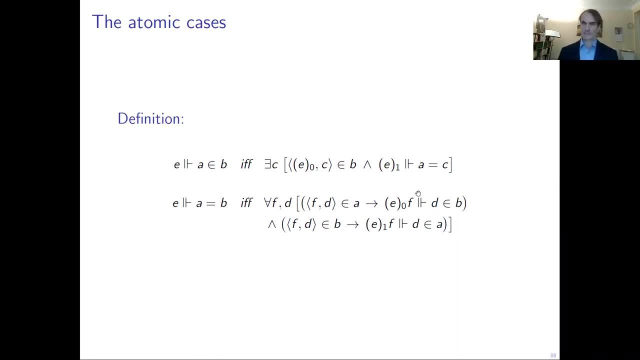 So you see, because, yeah, so this the equality appears on the right hand side And again the A appears that this must be a recursive definition, So it's defined by trans finite recursion. And then, similarly, for the A equals B. 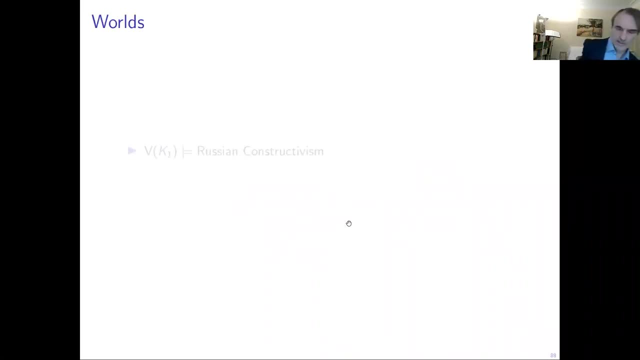 Okay, So that's the definition of this type of realisability, And it has very interesting consequences. So now you, most of the time people just use maybe one or two Of the PCAs, And if you use the first Kleene algebra, so this means Turing machine application, you get a world in which some of the principles that are cherished in Russian constructivism are valid. 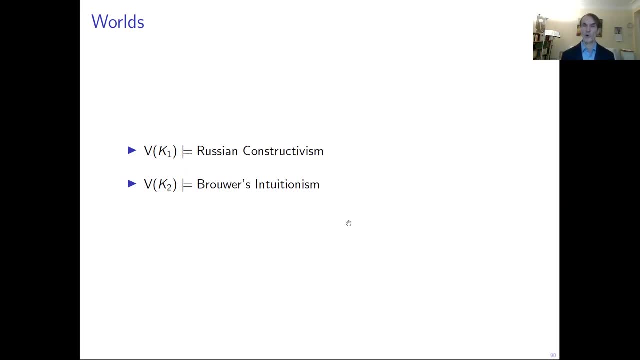 For instance, the Church's thesis would hold in this universe. So, all so, in this, internally in this world, in this world VK1,, all functions from the natural to the naturals are computable If, instead of K1, you take K2,, the second Kleene algebra. 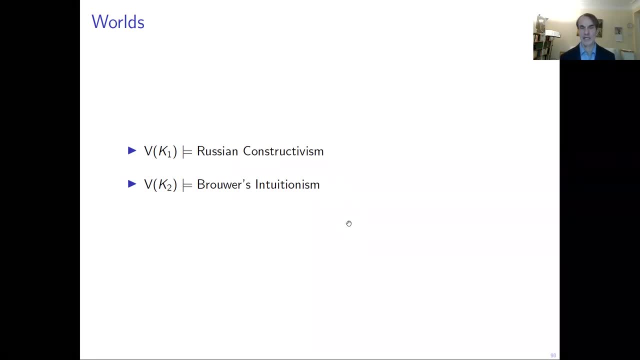 which is based on bare space and continuous function application, you actually get a world which is more adapted to Brouwer's intuitionism, For instance. many operations become continuous. But of course one could look at many, many more of these PCAs and find 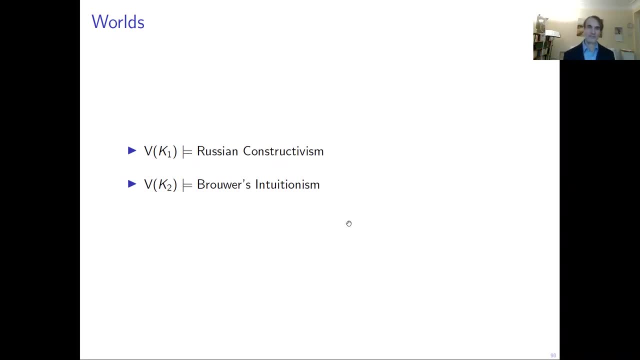 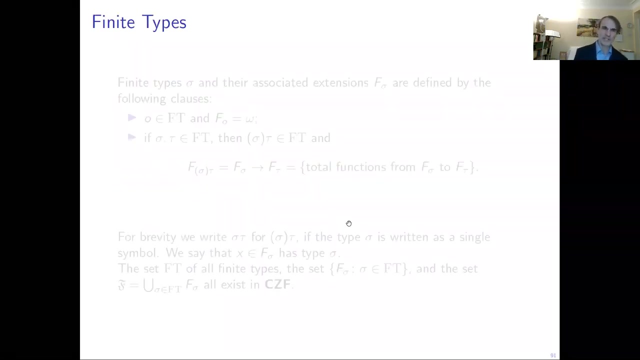 many more interesting worlds. I think this is one of the beautiful things about studying these realisability models: that you end up with so many different set theoretic worlds. OK, Now I would like to go back to the, to the Goodman result. So this was. 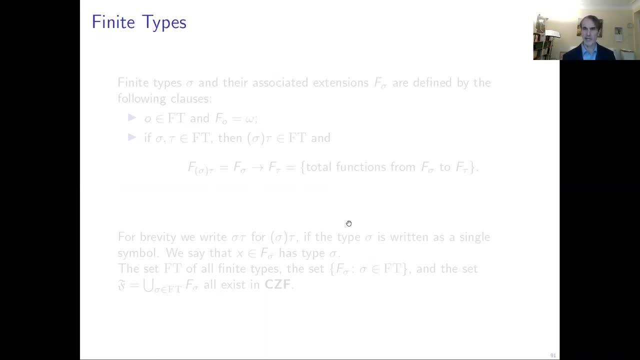 a conservativity result. Adding the axioms- the axiom of choice for finite types- doesn't yield new arithmetic statements, So just the definition here. So the finite types are. so this Ft here just defines the set of finite type symbols. So this O or zero is the lowest type. 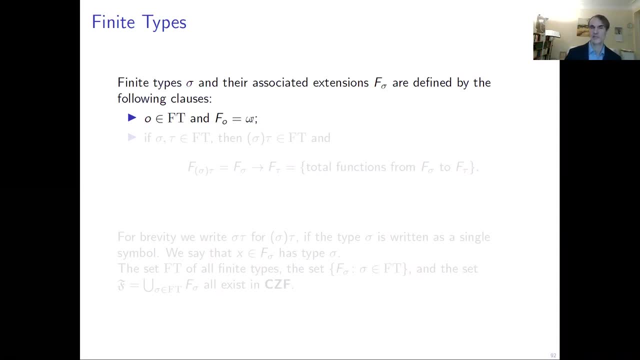 That's just a type of natural numbers or omega in the set, theoretic setting, And if you have two of these finite types, sigma and tau, then just writing sigma- tau. in this way here is another finite type And it denotes the the type of functions from F sigma to F tau. 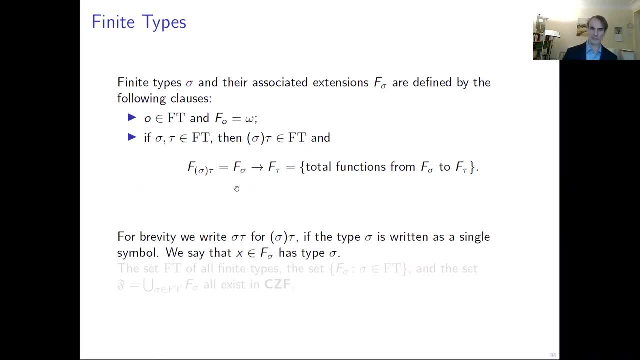 OK, And then in the future I'll just write sigma tau without the parentheses around it, And by Ft I'll just denote all the finite types. And just one remark: Where do the finite types exist? Well, for instance, the finite types exist. 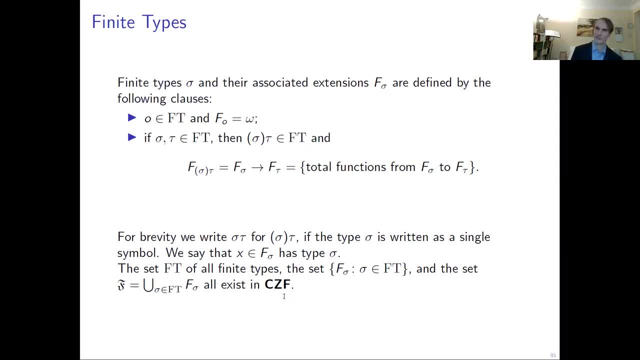 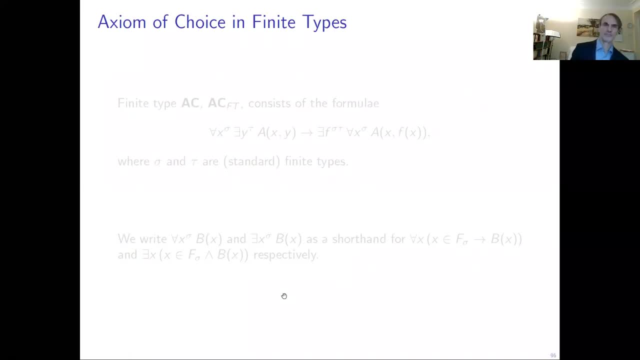 in constructive Sarmiello-Frank set theory, And of course they also exist in IZF. OK, And then. so here we have the, the choice axioms associated to the, to the finite types. So if you have a combination for all X sigma, 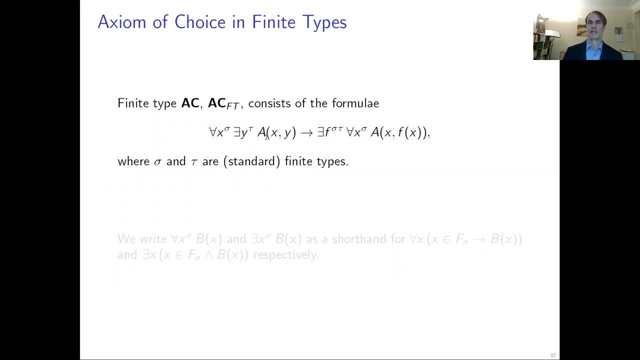 there's a Y tau AXY, Well then you should be able to extract a function out of it. namely, then there's a function of type sigma tau which takes an object X sigma into the type F tau, And we have that for all: X sigma AX. 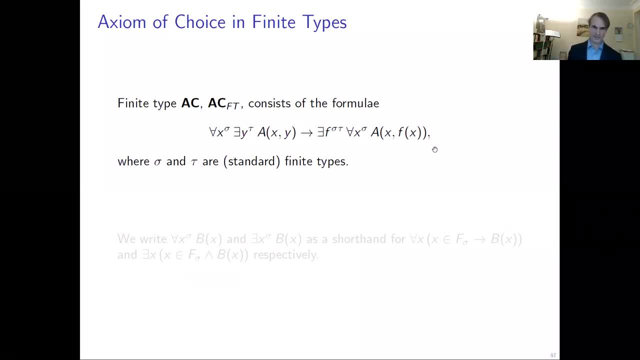 F, X holds. So these are these axioms of choice. OK, And so what happens is Goodman's result says: if you add these choice axioms to a higher type, heighten arithmetic, then no new arithmetic statements are proved. OK, The next thing. 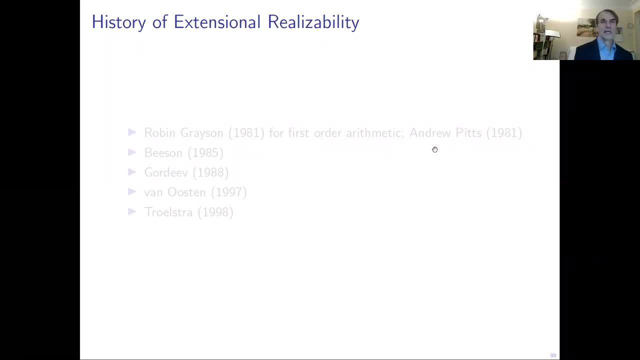 I'd like to talk about is this: generic realizability can be, in a certain sense, in a certain sense beefed up to what I'm going to, what I'm going to call extensional realizability. Now, extensional realizability has been studied before. 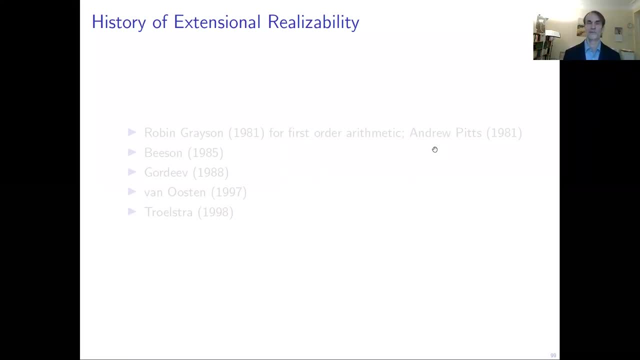 in connection with other notions of realizability, in particular a realizability for H A. So, for instance, Robin Grayson, I think is maybe the first reference that you find something like that. Interestingly, he was in Munster at the time. 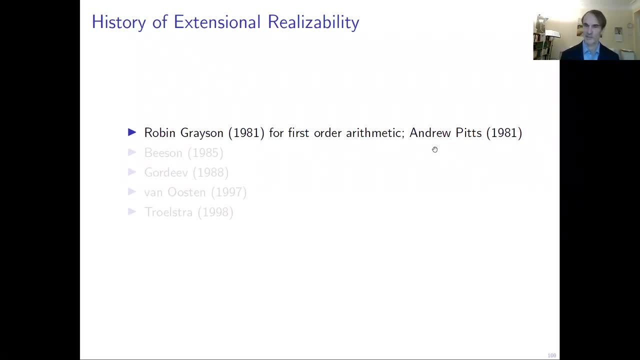 and I was a student there, so I had some contact with him at the time. Surprisingly, many, many years later, I use this stuff. OK, It was also used by Beeson, by Gurdjieff, by van Olsen and Tolstra. 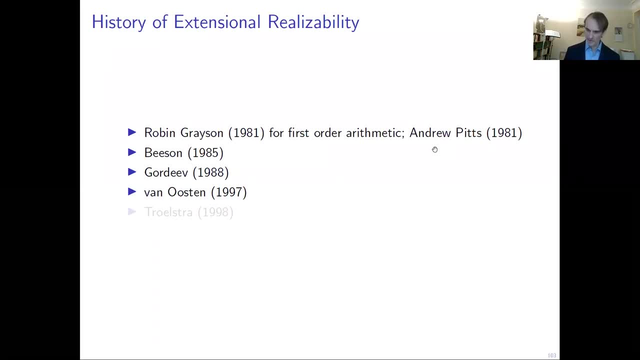 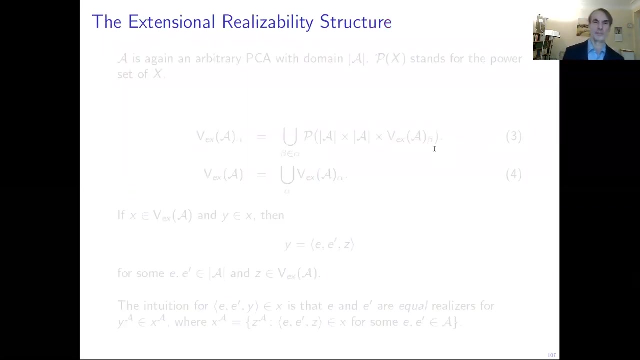 But I think it was never used for this type of generic realizability, for set theory. OK, Of course, it's a very natural step, And so this is now the joint work with Emanuele Fritaillon, And so the previous realizability structure. 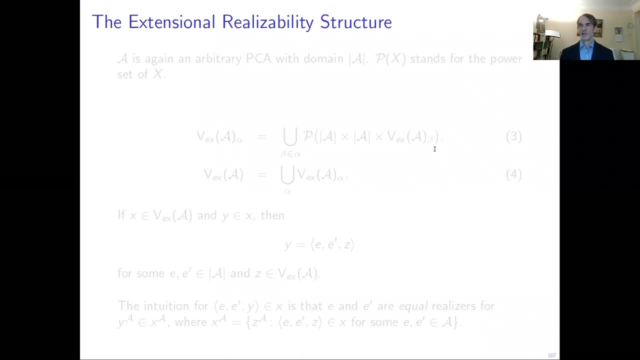 as I said, we would like to beef up to take care of realizing of more extensionality. OK, And so the difference now is: again we start as an arbitrary PCA. that doesn't change. but the realizability universe has another component, Namely 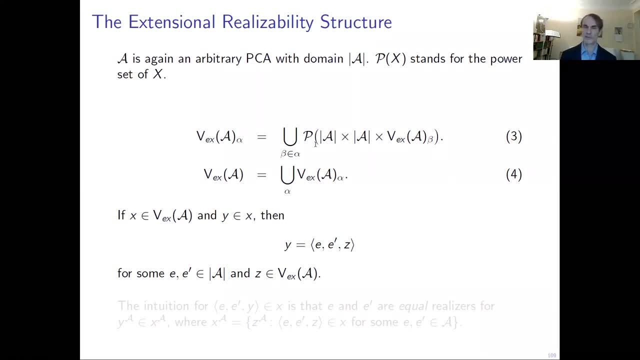 in the previous case, in the realizability universe, before there was only one copy of the domain of A, And here we have two copies instead, And so that's the main change, And what this means is, if you take an inhabitant of this universe, 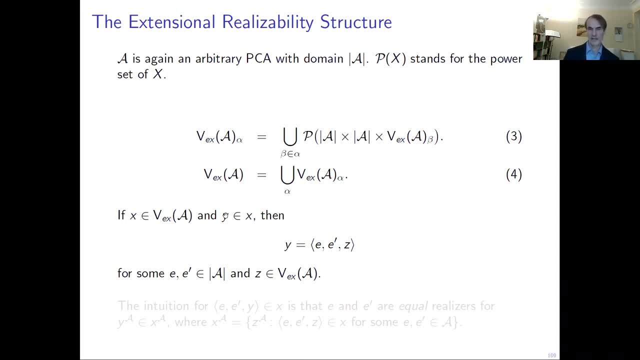 so let's call it X. and then the elements Y of this X are triples, But the first two components are from the PCA, the given PCA, and Z is another inhabitant of this world. And OK, And having now these 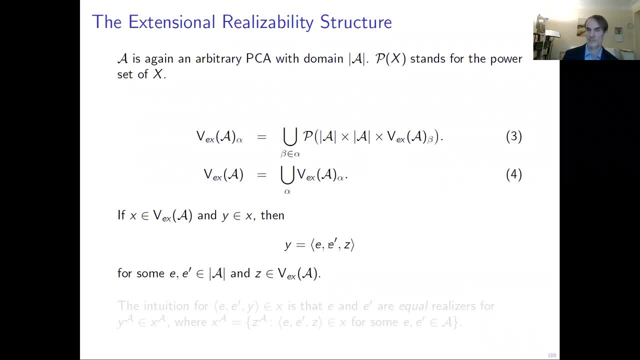 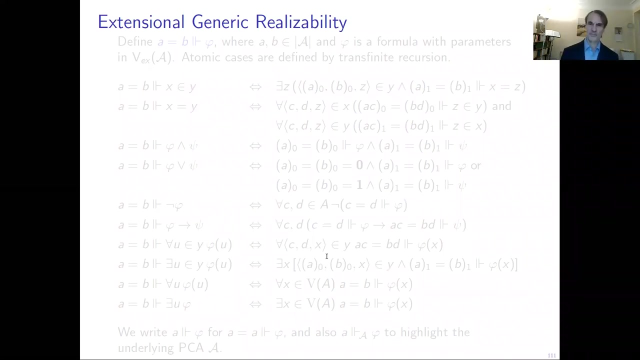 basically these two realizes. as an additional information, we will use it to express that E and E prime are equal realizes of something. And OK. So the realizability definition looks now more involved. The general pattern now is that instead- OK, I'll just flush the 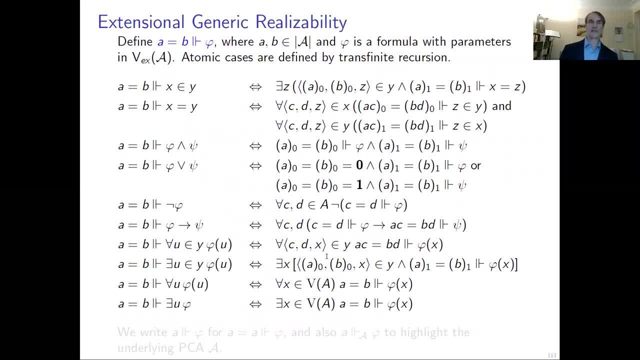 flash up the whole thing here. So, instead of having in front of this realizability symbol just having one realizer, we have two, basically, And what we would like to define here is basically the notion that at least A and B from the PCA. 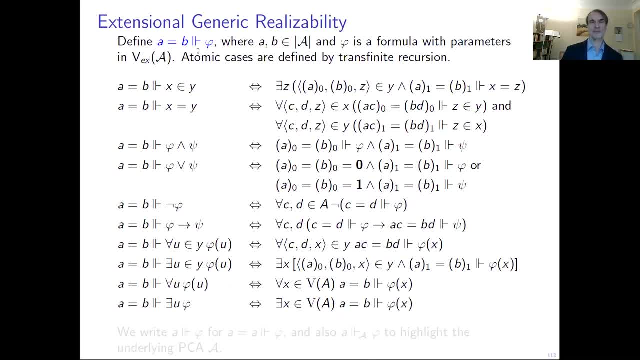 are equal realizes of some formula of set theory, phi. So phi is a formula of set theory which usually contains parameters from this extensional realizability universe. And there's an interesting thing, I think, here, And there's a connection to Martin-Loeff type theory. 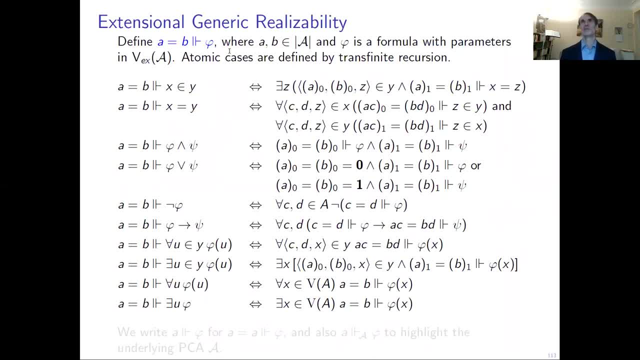 And Martin-Loeff type theory. if you view so, the denizens, the inhabitants of types, can be viewed as proofs, or also as realizers or as evidence. And in Martin-Loeff type theory we have the identity type and which has made 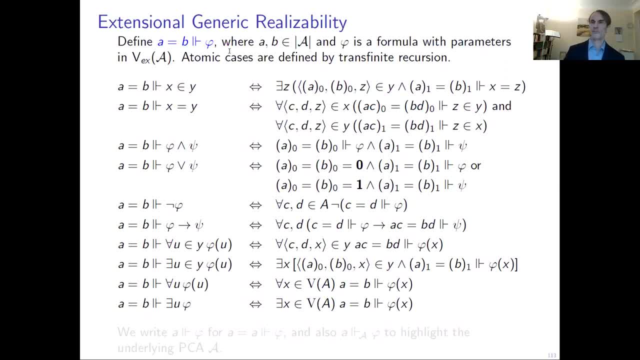 quite a splash over the last 15 years or so, And so, in a certain sense, there's a connection here. So we talk. we also talk about identity, in a certain sense, of realizers. Okay, Now what happens is one of the interesting cases. 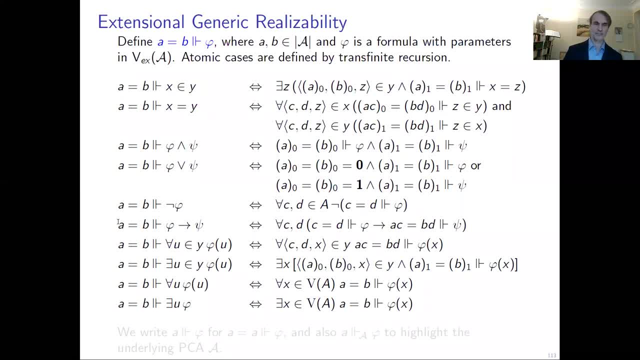 maybe I jumped to the case of the implication here. So here, what does it mean? that A and B are equal realizers of this implication, phi or psi? Well, it means that whenever we have equal realizers for phi, then applying A to C, 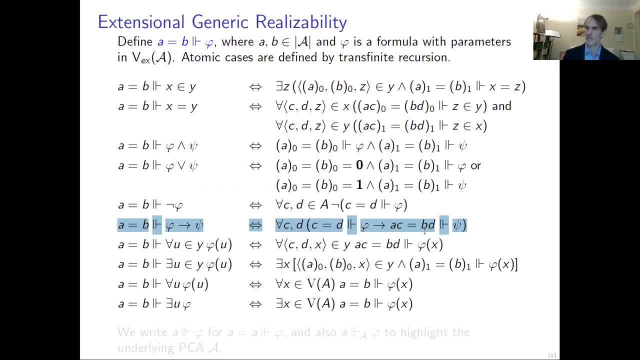 and on the other hand, B to D yields equal realizers for the consequent psi. Yeah And then. so that's the crucial part here, Whereas for the, I treated here the bounded quantifier separately. Now for in general. 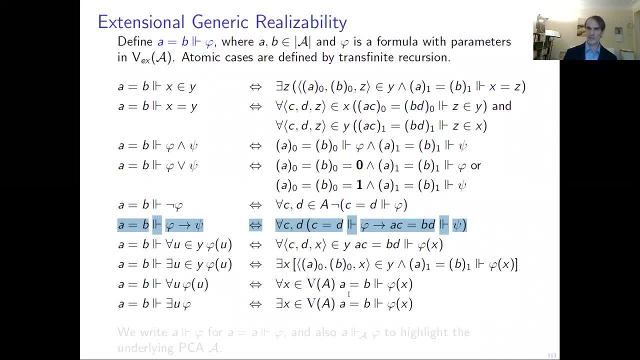 for the unbounded quantifiers. we have the same generosity here, namely that an equal realizer, equal realizers, for universal statement means just that these are equal realizers for any instance simultaneously. Yeah, Okay, So this is an extensional. 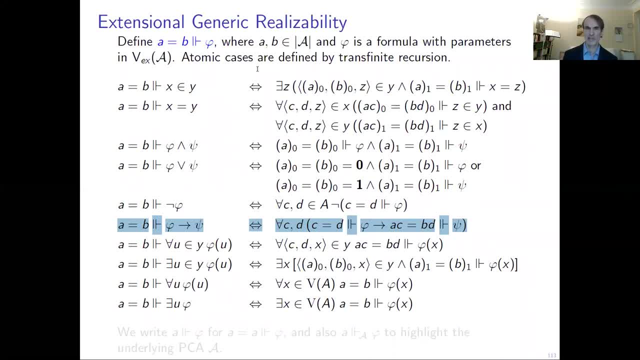 realizability or, more specifically, extensional generic realizability. Okay, And usually there's some convention here: instead of writing A equals A realizes phi, just write A realizes phi, And well, as I said, it's very interesting. 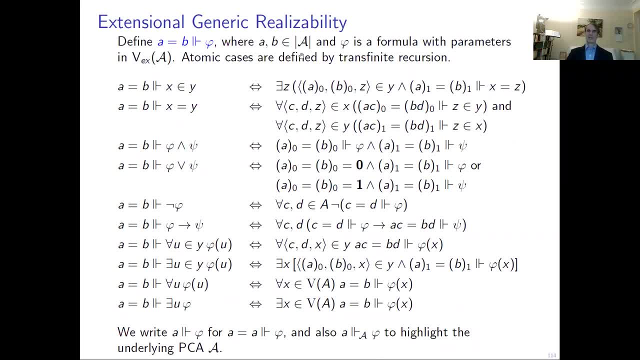 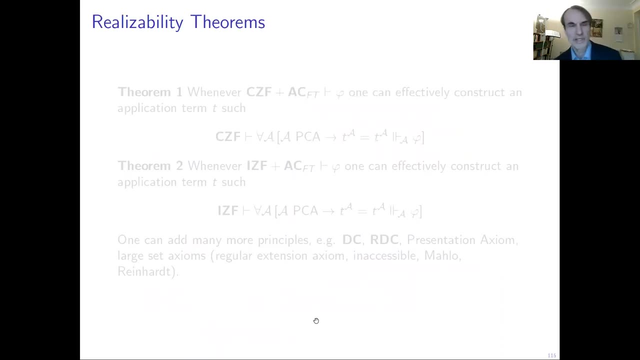 to study different PCAs here and to indicate the PCA associated with this realizability. sometimes use the subscript A here. Okay, Now what happens? What kind of realizability theorems do we get with this type of realizability? One thing is that. 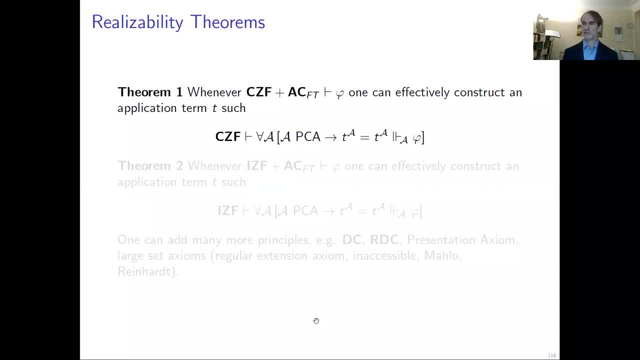 this realizability will realize the axiom of choice in finite types. So the situation is maybe starting with the constructive, similar set theory if you add to it a CFT and you prove- yeah, and you prove any set theoretic statement. 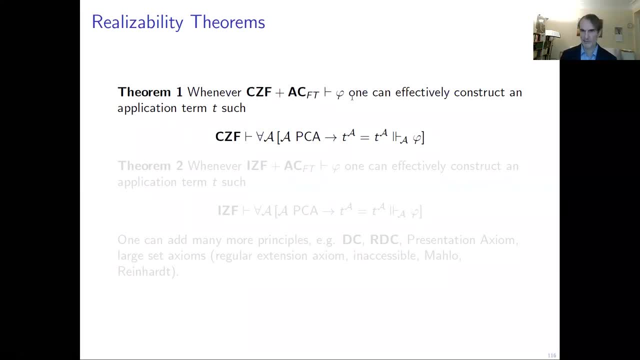 and then from the proof one can effectively construct an application term. So an application term is a term of the theory PCA, the abstract theory PCA, such that CZF proofs for any PCA A. if one evaluates the term in that PCA then TA equals TA. 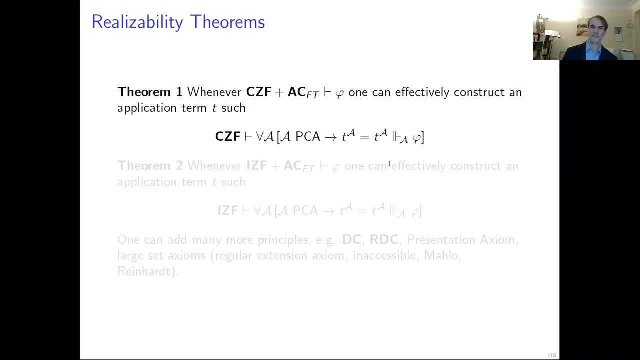 is a realizer for phi. So this goes to say that this holds in a very, very uniform way. So the realizer that we construct we just get out of the out of the proof, It's an effective construction of the realizer. 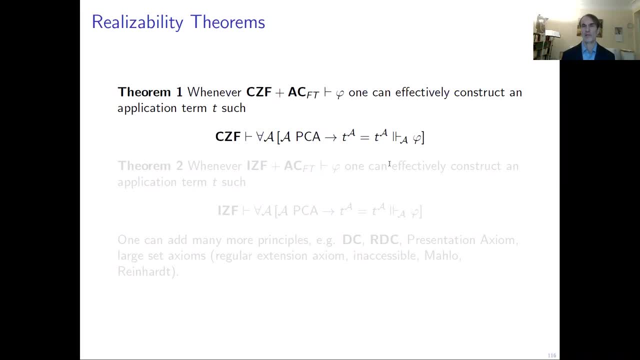 We do not say there exists some realizer, but we actually have a particular term And this term then provides a realizer for any PCA. Of course the term has to has to be evaluated in that in any given PCA Okay. 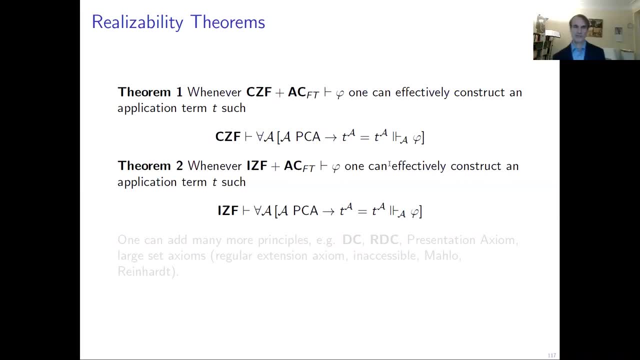 And the same result you obtain if you do. if you do the construction with IZF is the same And moreover, of course these are kind of very important theories, CZF and IZF, but you can add tons of other stuff and get. 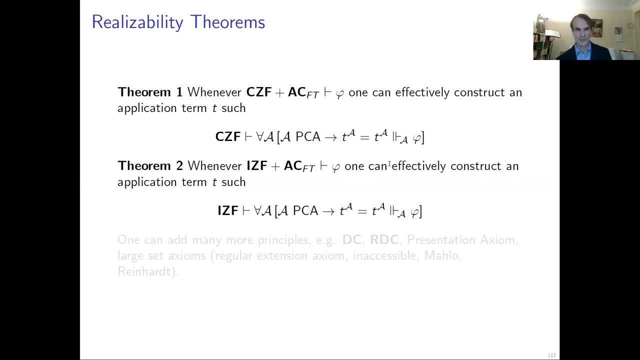 a realizability theorem. So for for any of these theorems, you can add principles like certain choice, principles that are okay in intuitionistic context, like dependent choice, relative-wise dependent choice, even the presentation axiom. You can add large set axioms. 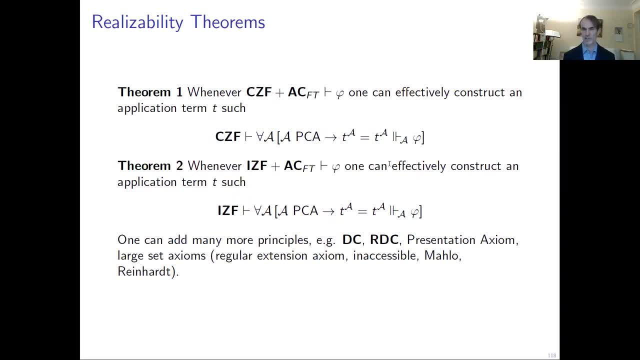 and then you would get the same result. Okay, So that's very nice. So you? so this kind of realizability allows you to realize these finite type choice axioms. And then the idea is to combine it with the Goodman theorem, and then 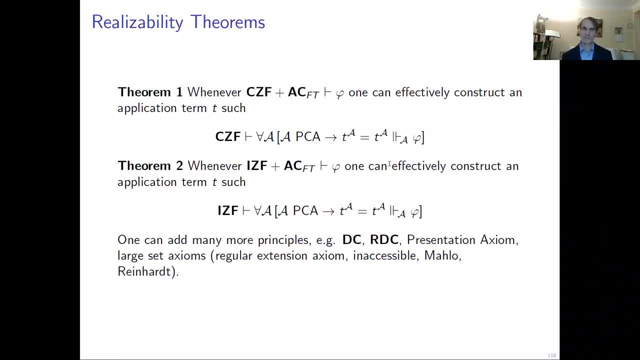 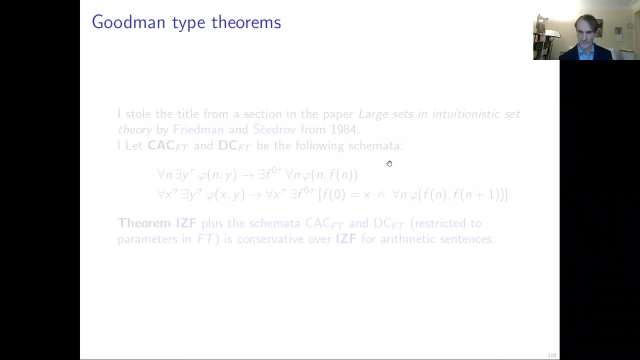 you can get the same result. And then the idea is to combine it with the Goodman machinery. And another confession: I stole the title for the talk basically from a section of a paper by Friedman and Shadroff, But the paper is called Large Sets. 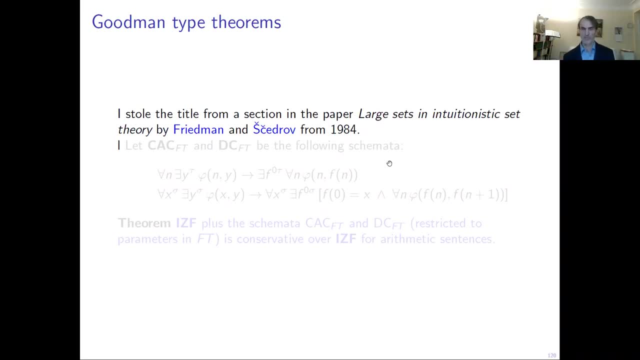 in Indiginistic Set Theory And they also studied some choice principles in finite types. Yeah, Maybe they studied special cases. So the first special case of the CAC stands for countable axiom of choice in finite types. So here you have a combination. 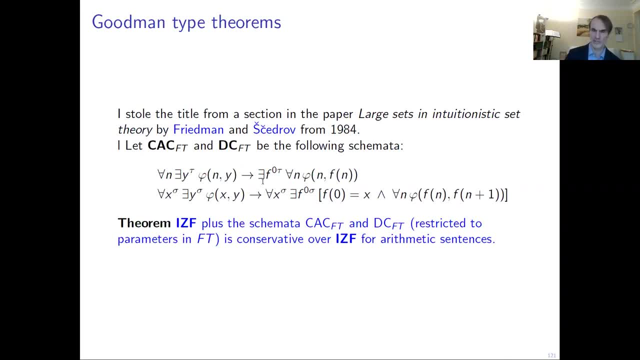 for all n, n is ranges over naturals. There's a y of type tau, phi and y. Well, you have a y sigma, You find a y sigma, so that phi, x, y holds. Then, given any x sigma you can produce. 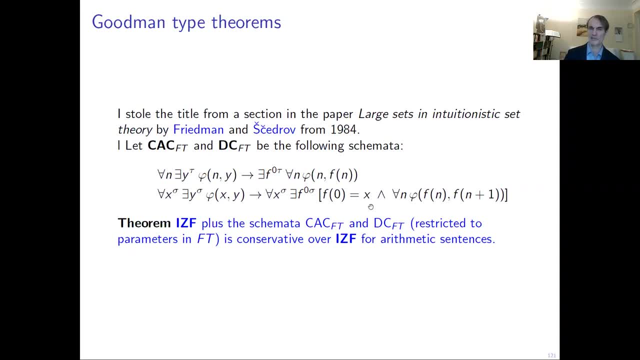 an omega sequence given by this function f here, So that f, 0 is the given x And for all n, phi, f, n, f of n plus 1 holds. And then they these principles to, for instance, to i, z, f. 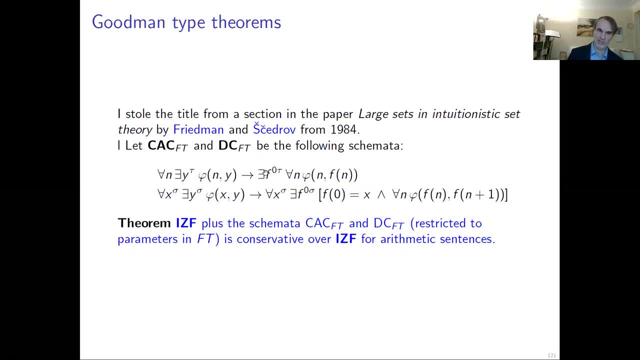 you do not generate new arithmetic statements. So now these are very special cases here And basically to show this, you only need some kind of, you only need to work with the, basically a form of 1945, and then you can prove all the finite. 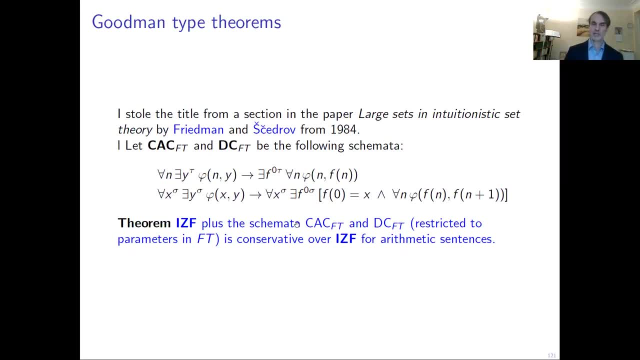 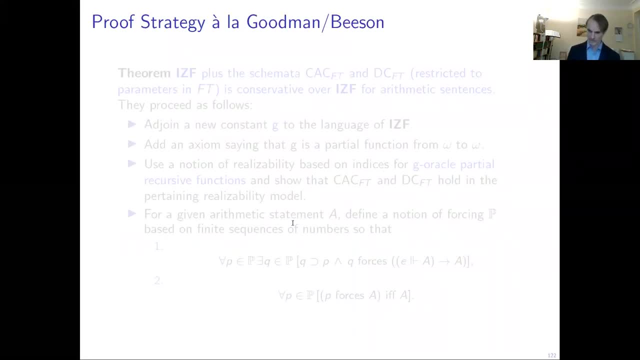 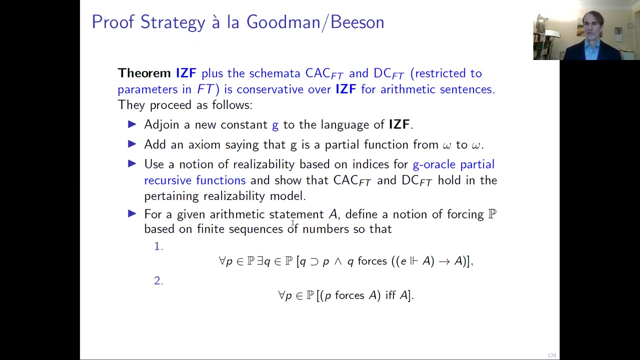 type actions of choice, And you can combine it with the Goodman machinery to get conservativity. And just a reminder of the Goodman machinery, just very, very briefly. So the Goodman machinery consists of: you basically do an extension of the first clean algebra K1.. 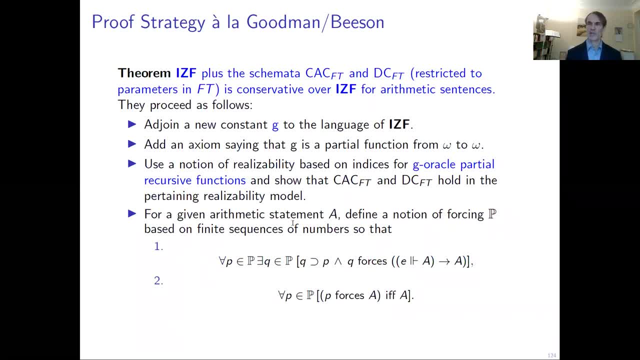 So instead of Turing machine application, you do Turing machine application, where the Turing machine has attached to it an oracle, basically, And if it's defined for your question, it gives you an answer and otherwise nothing happens. And then, basically, you do, you come up, 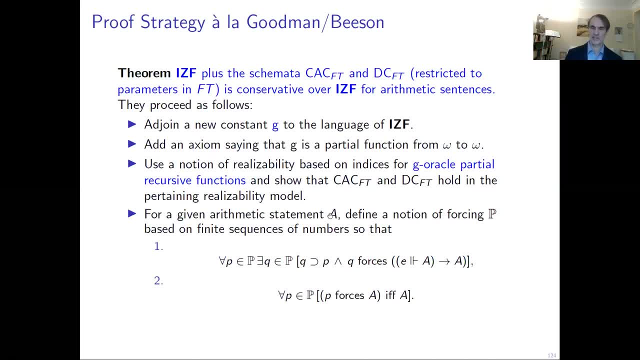 with a PCA that has this oracle which enshrines this, which is based on finite sequences of numbers. So basically, what holds? if you take any, any P in the forcing set P, then you can find an extension and the extension forces that if E realizes A. 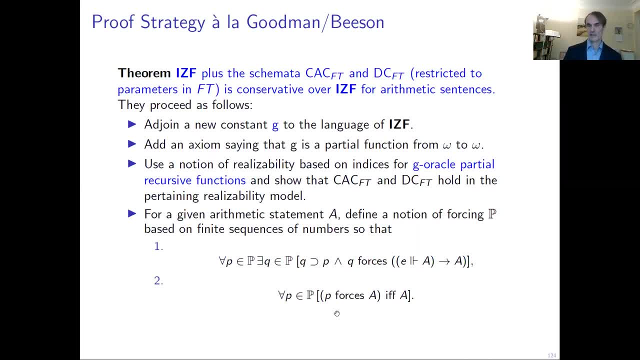 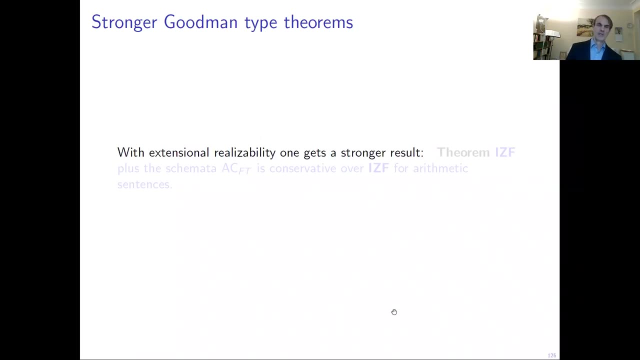 then A is true And, moreover, you have a certain function that is forced, then it's true. And so this machinery was used by Goodman and also by Beeson to get this kind of conservativity result. And yeah, and now is the. and combining this now. 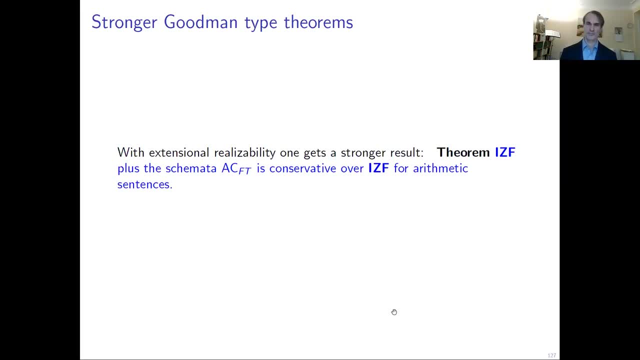 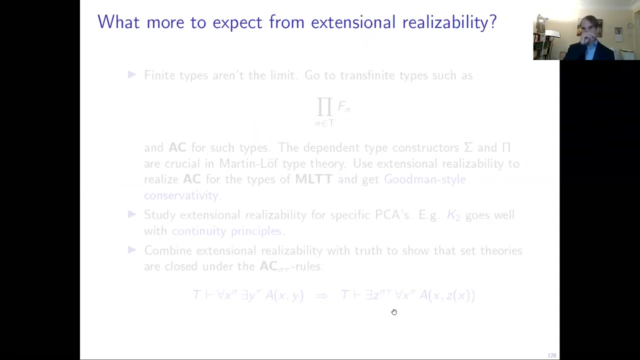 with the generic extensional realize ability you get that IZF. the actual choice for finite types is conservative over IZF for arithmetic sentences. Okay, So this now is my last slide here. This is: I think this is just the beginning of what you can. 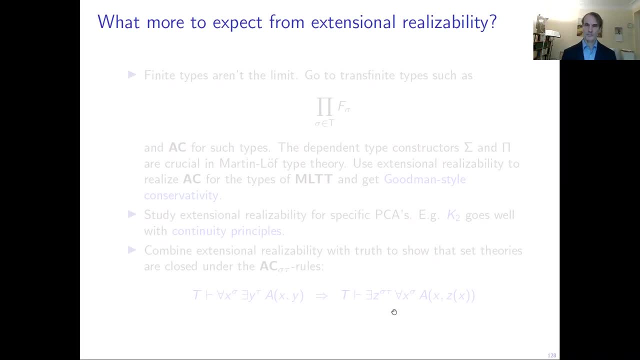 do with generic extensional. realize that the new choice principles we added to intuitionistic set theories were choice principles for finite types. But why stop there? Actually, you can go to transfinite types. Already did this in his paper on the infinite, So you 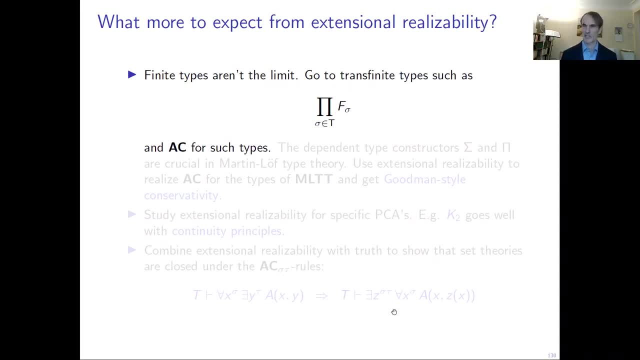 can for finite types into one type, like you can do in Martin love type theory. In Martin love type theory you have these dependent type constructors, sigma and pi, And then the conjecture is that all the types are finite types with extensional realize ability and 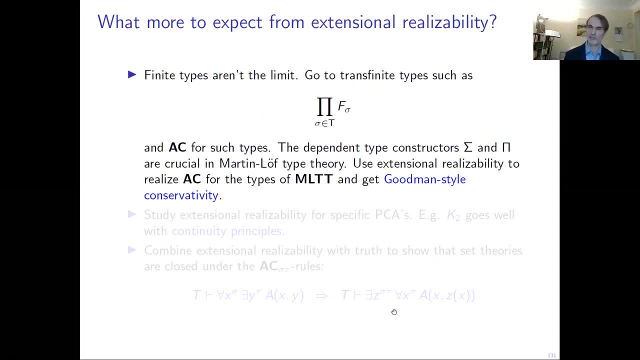 the good man machinery. Yeah, So this, there's much more here, And already it has been shown, actually for the first time, that you can add for all of these types an axiom of choice, like it holds in Martin love type theory, And then you 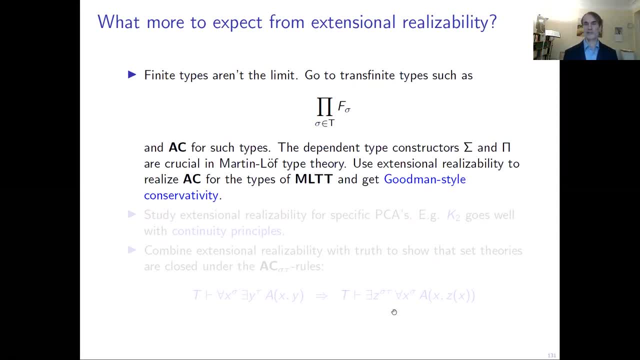 get conservativity, and what different PCAs give you, In particular the PCA K2, based on bare space and continuous function application, is very nice. if you want to get continuity principles And so much choice, can we add? So this could be explored Furthermore. 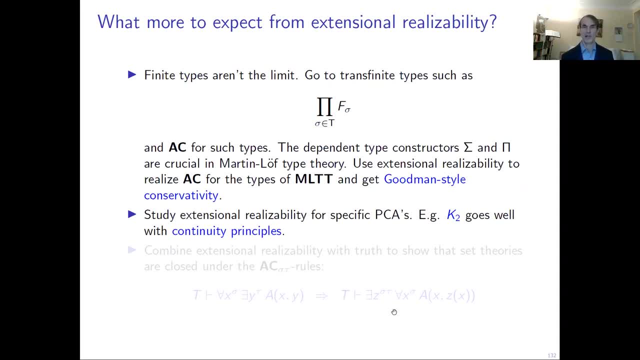 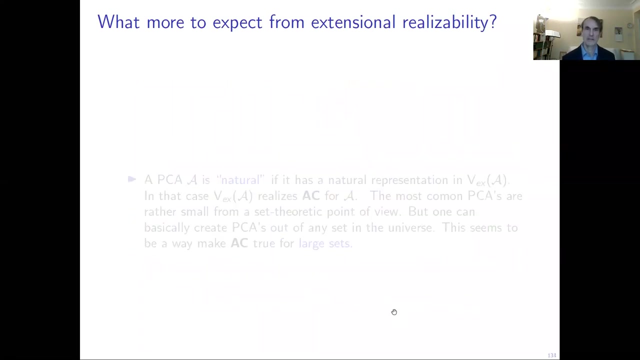 there is a way of getting meta mathematical results about derived rules. So you can. and one projection is that if you want to get the meta of any set theories under the AC, sigma, tau, rules for finite types, sigma and tau, And the final thing is I: